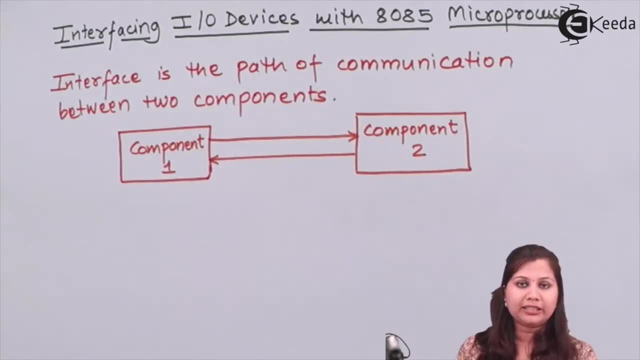 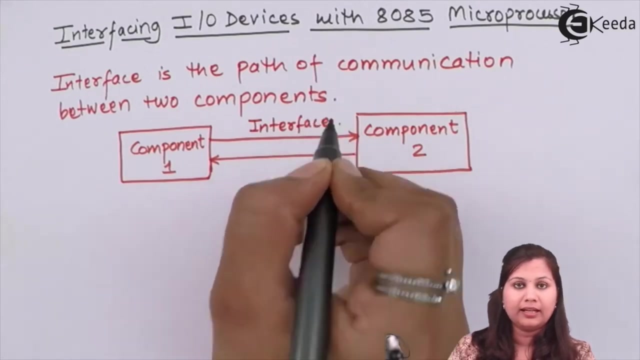 number one. So any transfer of data, that will be called the communication between the two components. so the path which is providing the data transfer between two components, that is called the interface, And interfacing it is defined as a technique of connecting the two components. 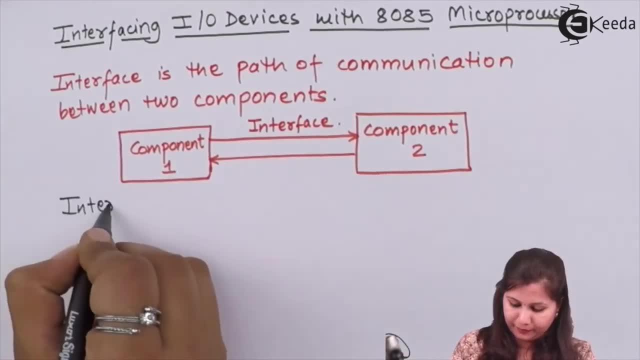 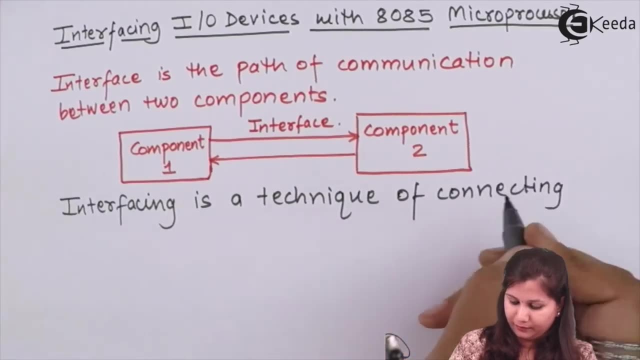 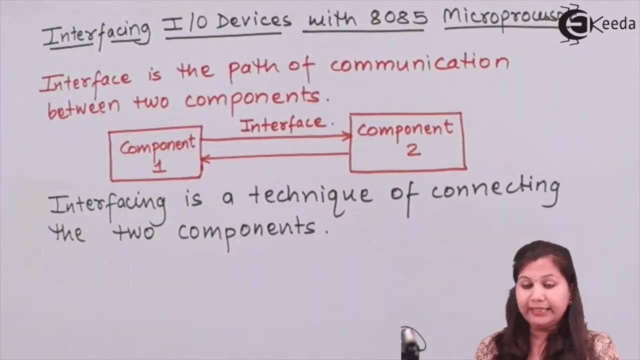 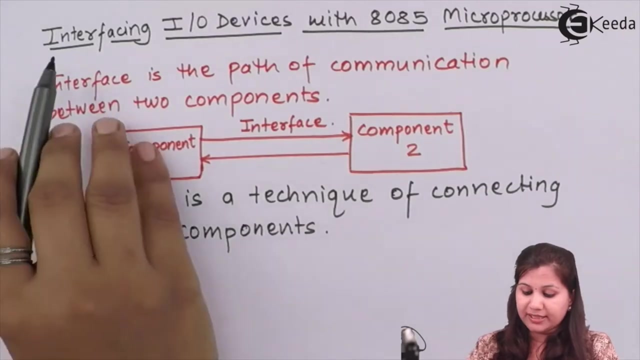 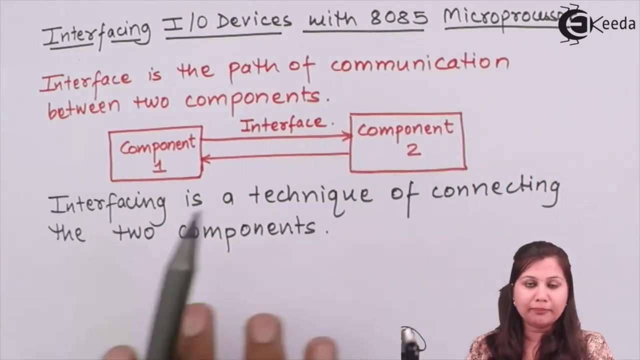 components. So interfacing will be defined as the technique of connecting the two components, that how these two components are communicating with each other. So here we are studying the interfacing of the input output devices with the 8085 microprocessor. So out of these components, one component will be our microprocessor and another component 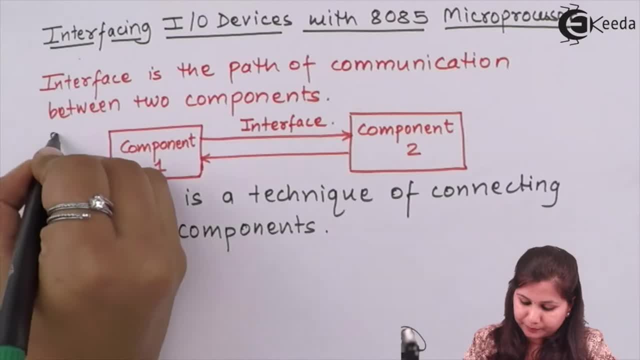 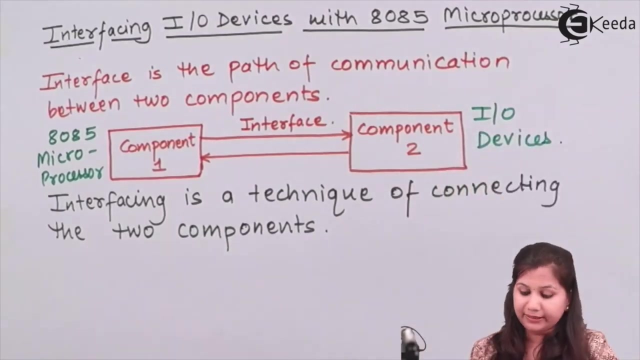 will be the input output devices. So here we will study that: How the input output devices- they are communicating with the 8085 microprocessor, What is the technique used, what are the types of interfacing there and what addressing is used for connecting the input output devices with the microprocessor. 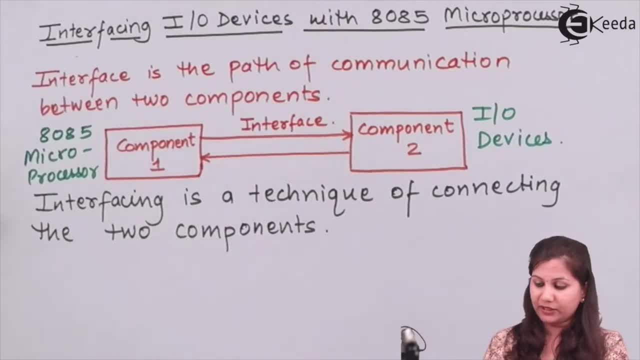 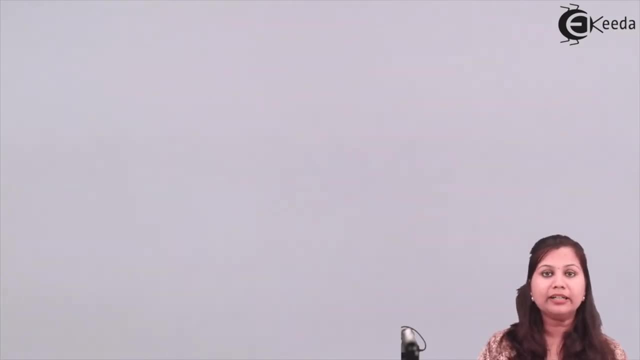 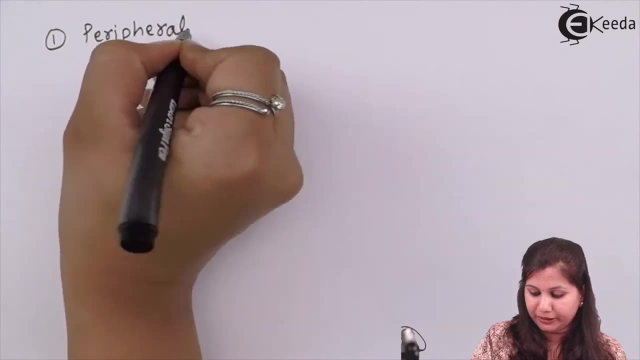 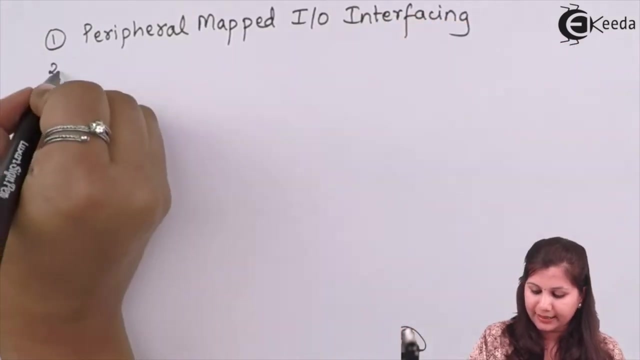 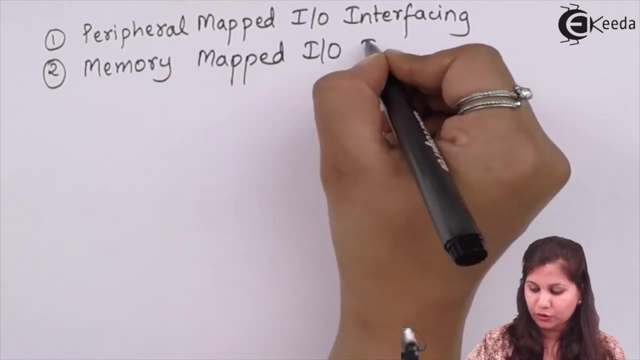 So let's start with the interfacing of input output devices with 8085 microprocessor. The input output devices. they can be interfaced with the microprocessor In two ways. first is peripheral mapped input output interfacing And second is memory mapped input output interfacing. 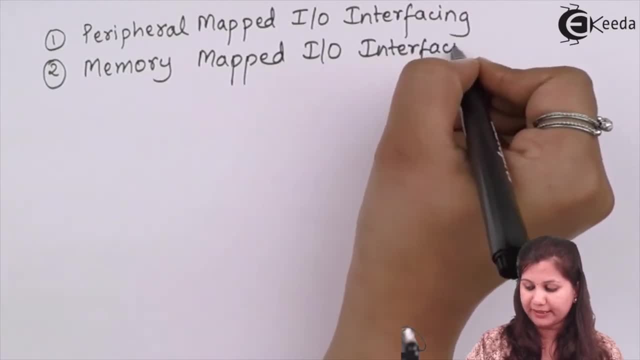 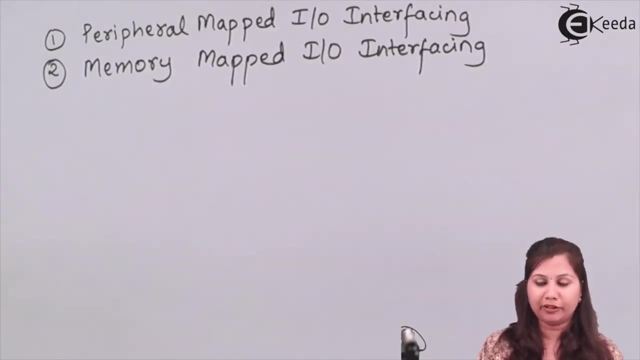 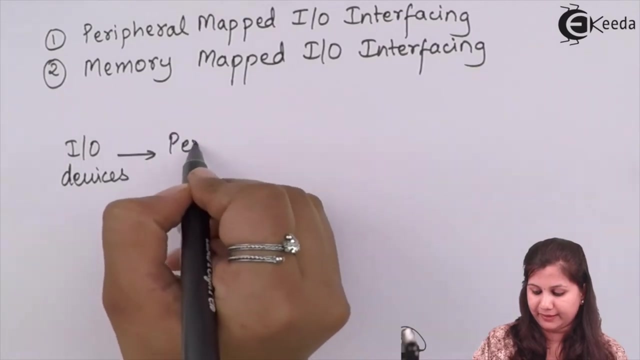 So we can say that there are two types of input output: interfacing: peripheral map and memory map, The input output term, It is also known as the peripheral. So whenever we are using the input output devices, we can also use the peripheral devices. 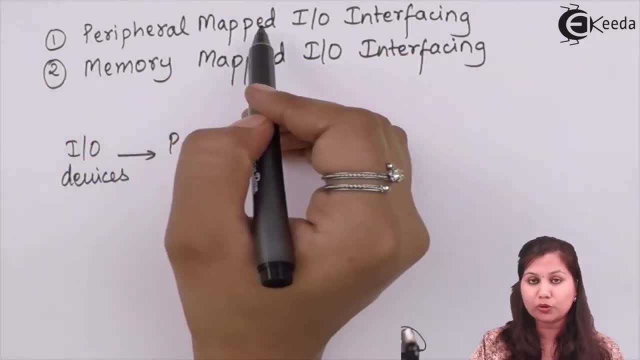 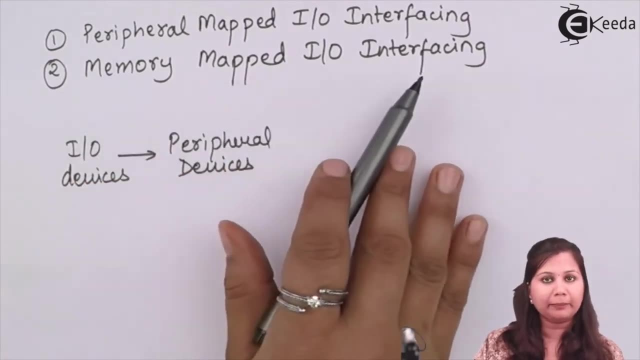 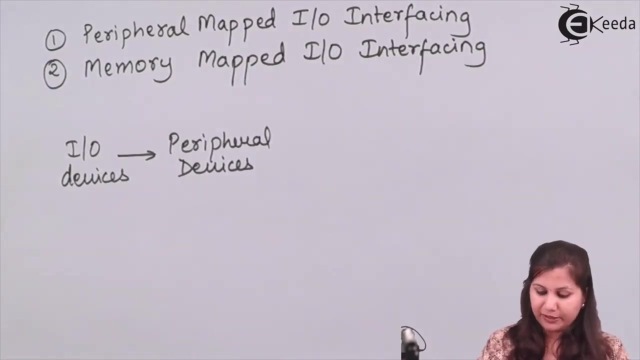 So this peripheral map input output interfacing- it can also be known as the input output map input output interfacing. and another type is memory map input output interfacing. So let us study These two types of input output interfacing. First, we will start with the peripheral mapped input output interfacing. 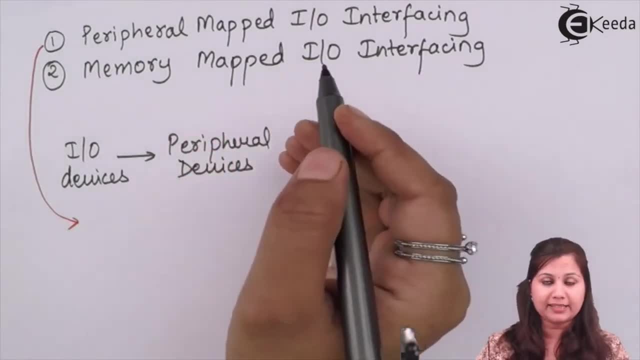 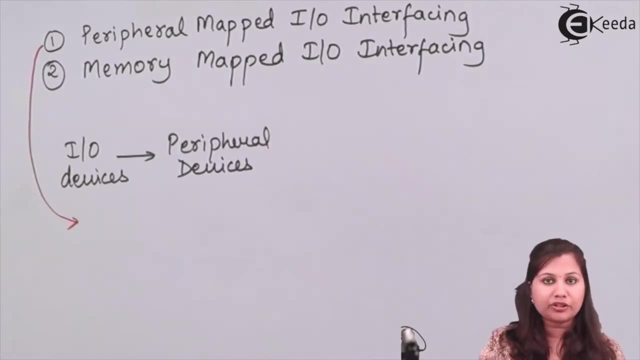 In this type of interfacing, the input output devices. they are treated as the input output devices also, not like the memory chips. So whatever functions are involved with the input output devices means whatever operations the microprocessor performed with an input output port, same functions will be performed. 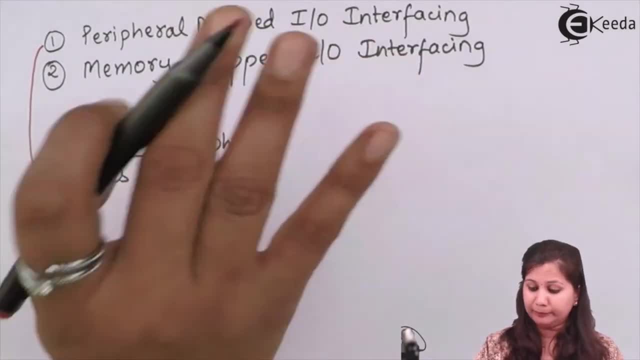 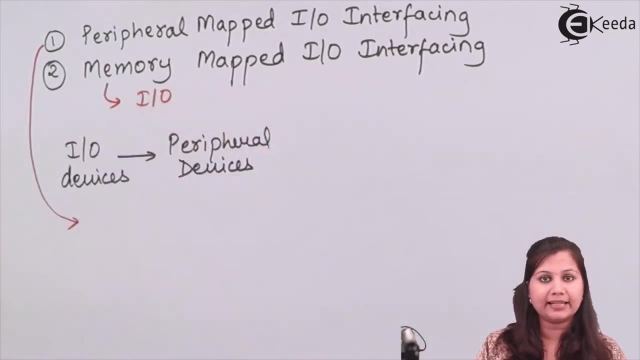 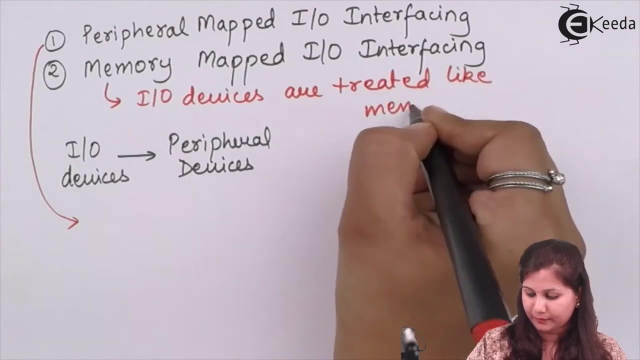 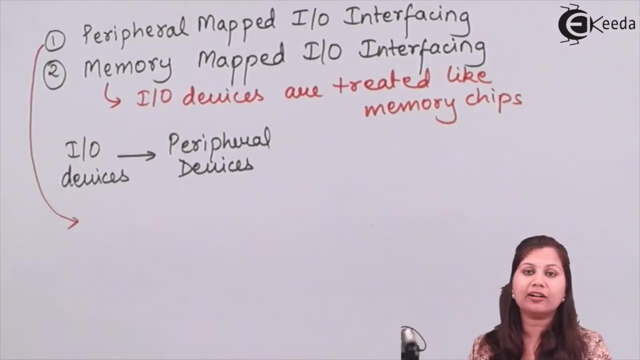 with in this interfacing Okay, Whereas in memory mapped input output interfacing the input output devices, they are treated as like the memory chips. So we can say that in peripheral mapped input output interfacing the input output devices they are not treated like memory chips and they will be treated just like the ordinary. 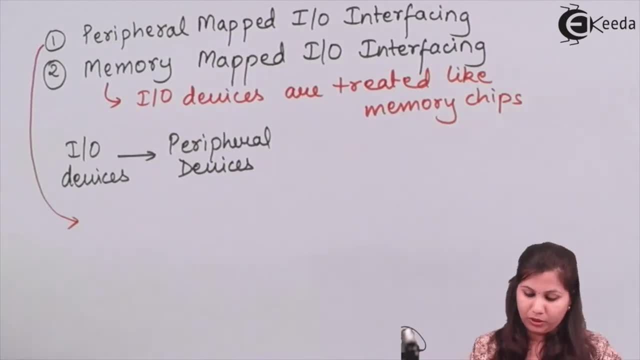 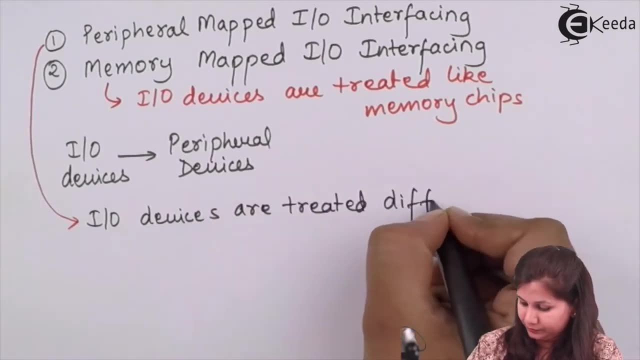 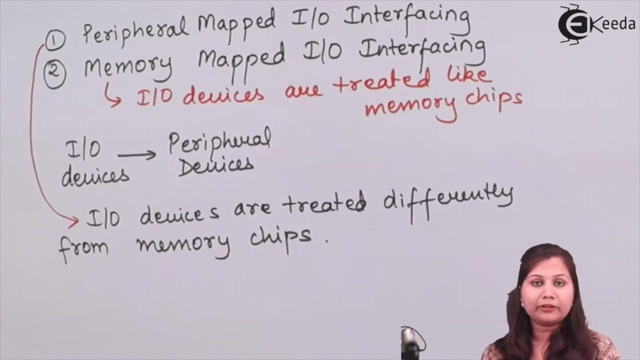 input output devices. So if I enter into the intake, So that means, let's say, two crying different input output ports. Now, when the microprocessor it is communicating with the input output devices, data transfer will takes place. Means microprocessor, it will either read the data from the input output ports or it is. 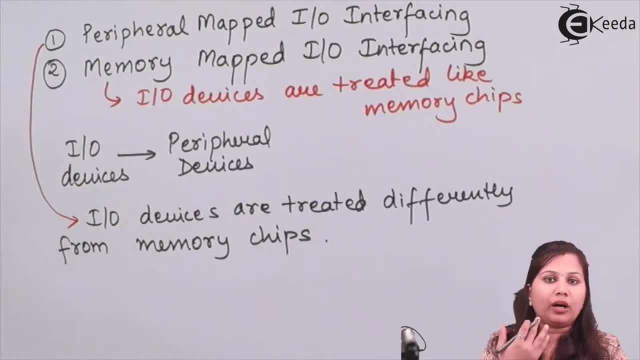 going to either write the data into a 200- muito clock, So in this scenario we can call it as micro processor. it will be transfer back to the input output ports. Neither are from the LAN, However, the data will transfer to the hotspot. 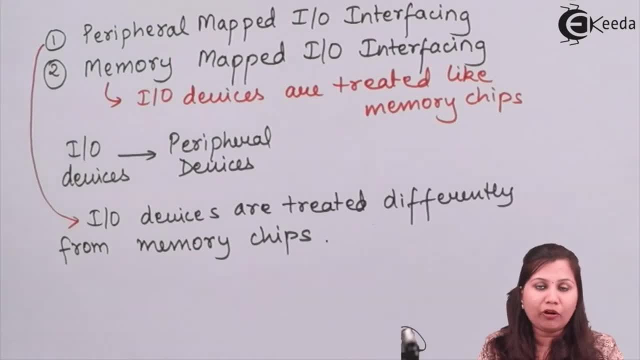 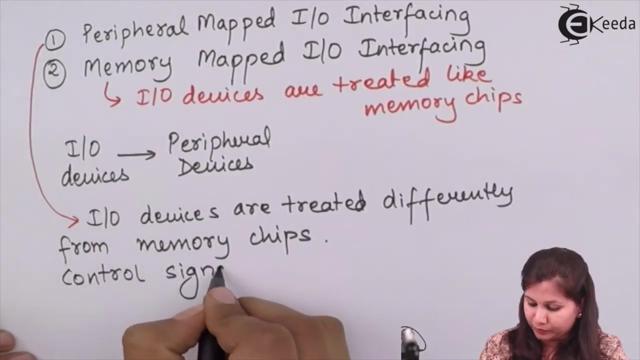 to the input output ports. So for reading and writing operations the microprocessor will provide the control signals. So in case of peripheral mapped input output interfacing the control signals are related to the input output operation. So in microprocessor 8085 we are having the 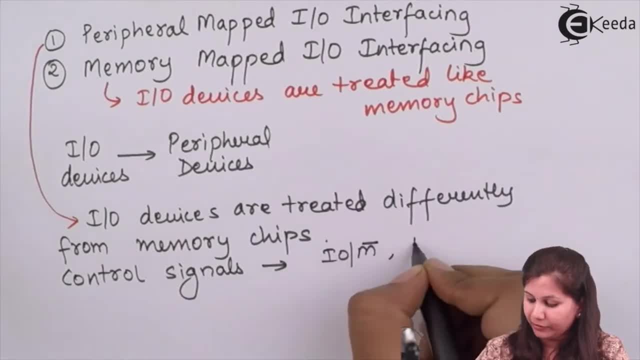 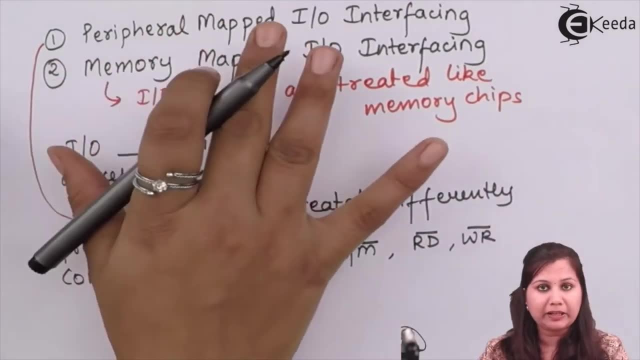 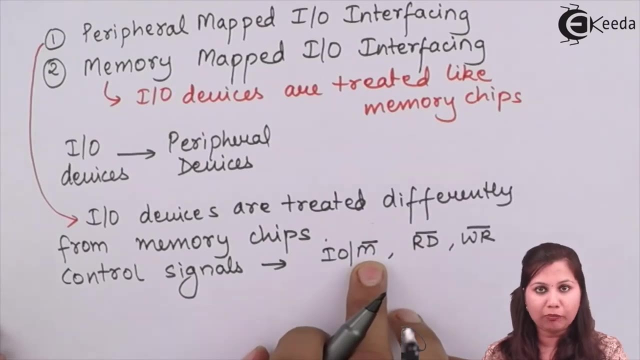 control signals- input, output and memory and read, write. So because control signals, in this case peripheral mapped input output interfacing, they are related to the input output operation. So here this will act as the input output signal: read and write. they will be combined. 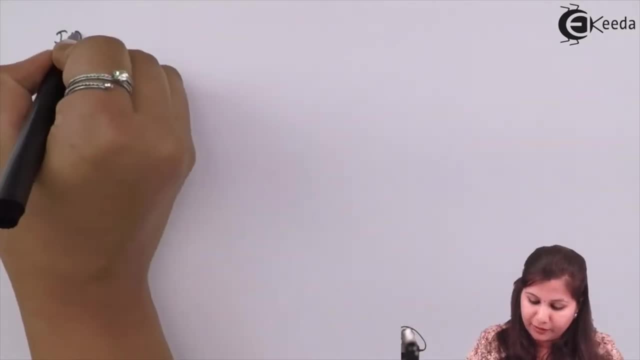 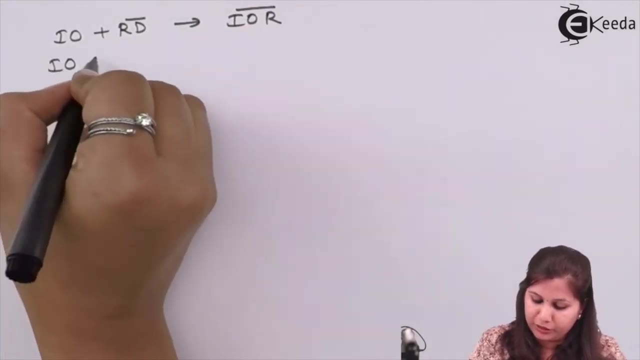 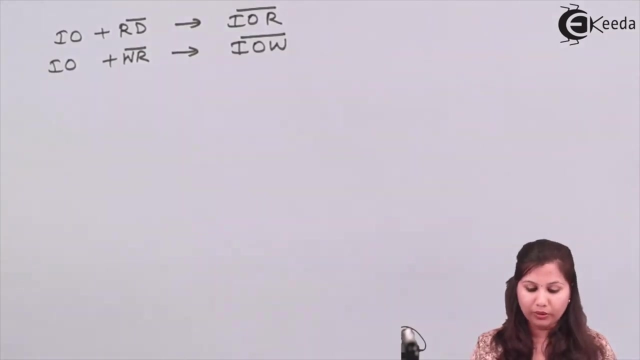 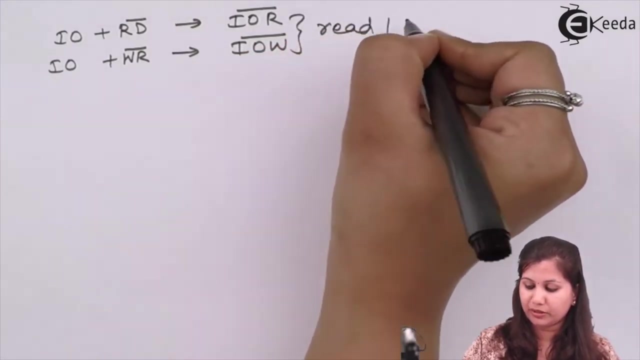 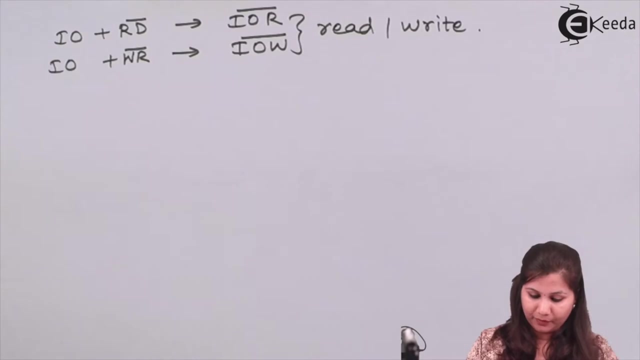 to form the two control signals. when input, output and read is combined, it will form IOR, and when input, output and write is combined, it will form IOW. So these two signals control signals. they are used for reading and writing from the input output devices. So let's see. 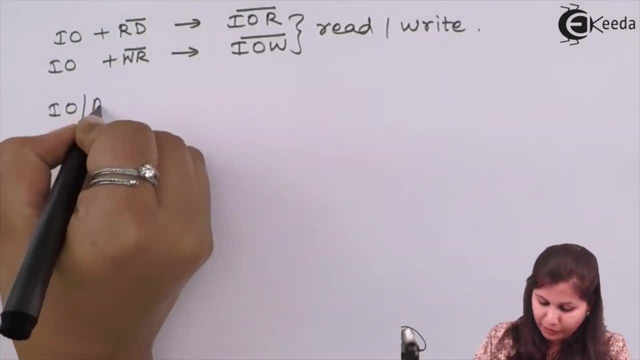 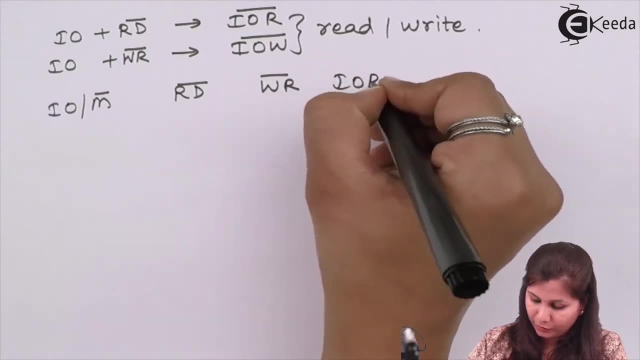 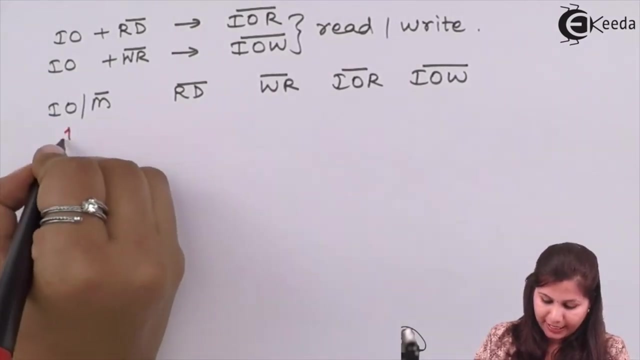 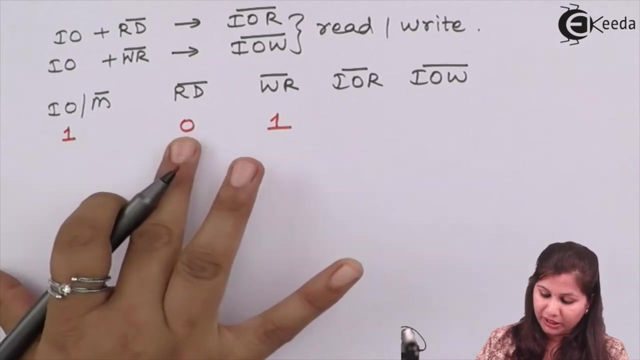 that what will be the status of these signals when the input, output and memory signal, read signal, read signal And write signal, IOR and IOW. So when this input, output and memory signal, it is at logic 1 when read is at logic 0 and write is at logic 1.. So when these two are combined means. 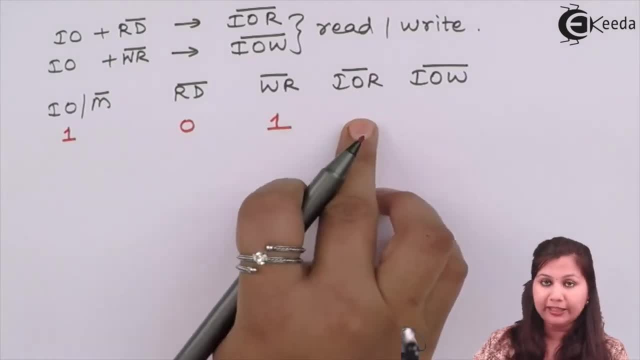 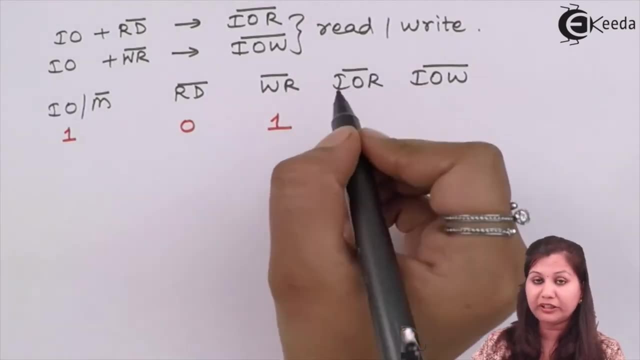 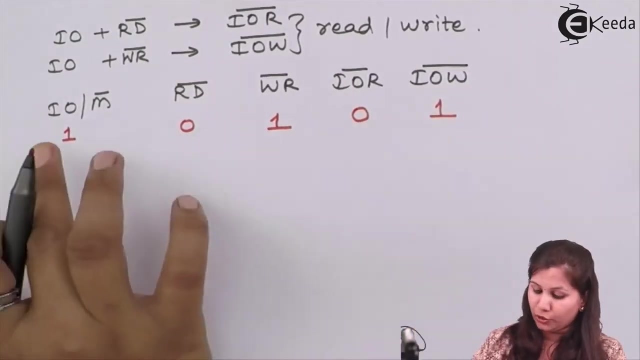 read is activated and input output is activated, IOR will be activated because this signal is having a bar over. it means it's an active low signal, So it will be active when its value is 0. it is inactive, So its value is 1.. So when 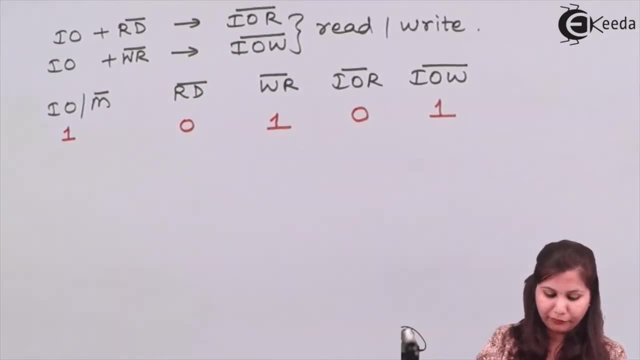 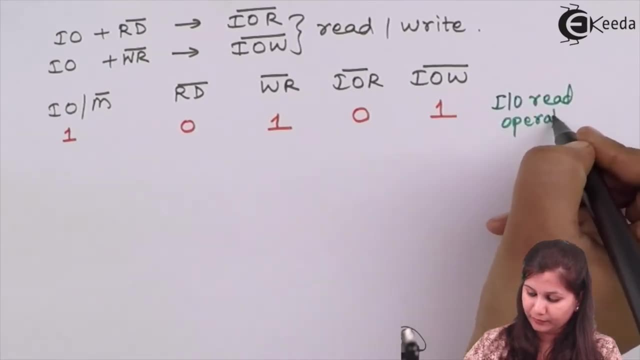 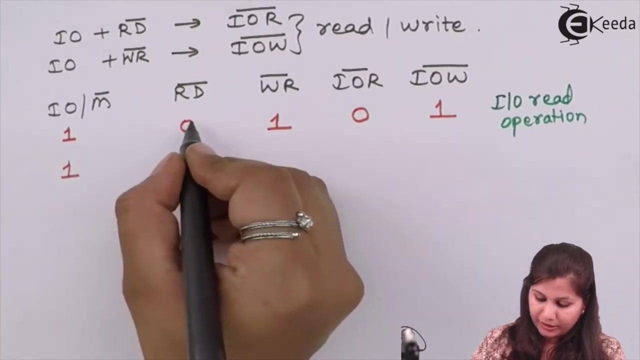 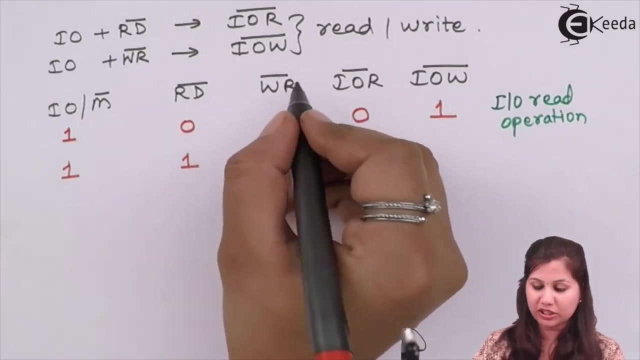 this is the status of the control signal. the operation performed will be the input output read operation. Next, if the input, output and memory it is at logic 1, read is at logic 1, write is at logic 0.. Send signal: read is at logic 1, read it means write is activated. it is also active low signal. 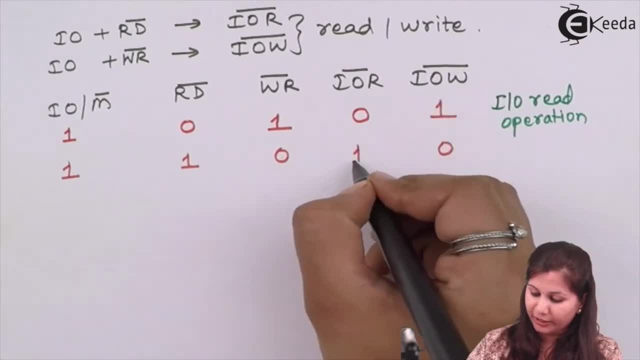 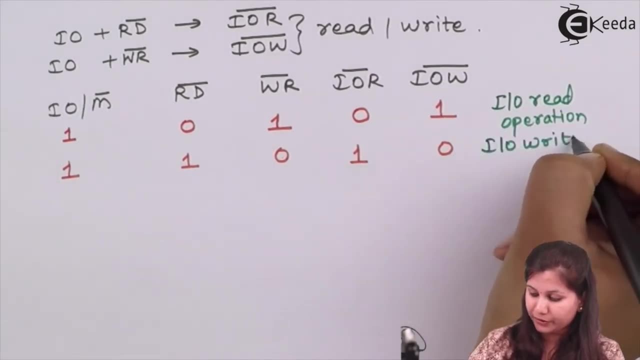 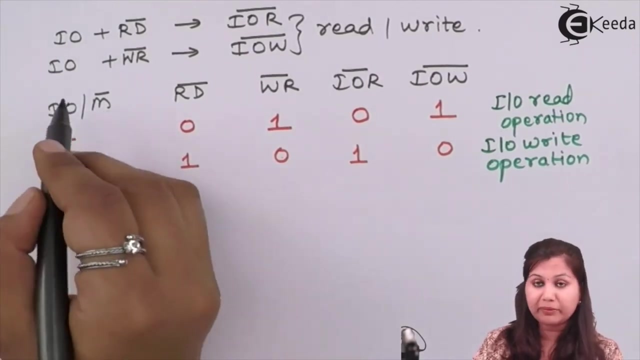 So in this case IOW will be activated, IOR is inactivated. So the operation performed is the input output write operation. Okay, Now here. if the value of input output and this signal it is 0, it means input output is inactive, memory is active. 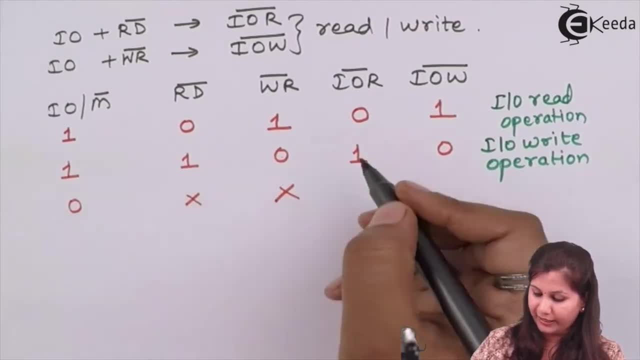 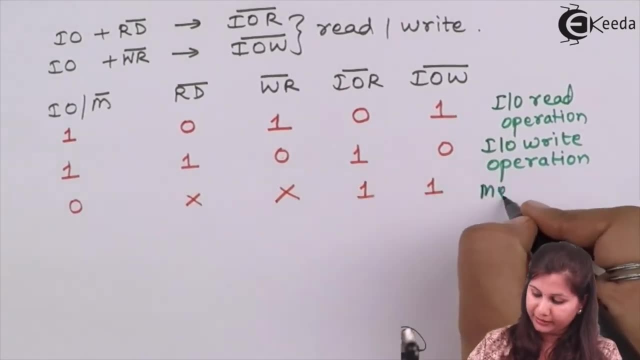 So whatever will be the status of this read and write and IOR is at 1, IOW is at logic 1, the operation performed will be either a memory read or write operation. Now here, because the input output devices, they are treated as the general input output ports. 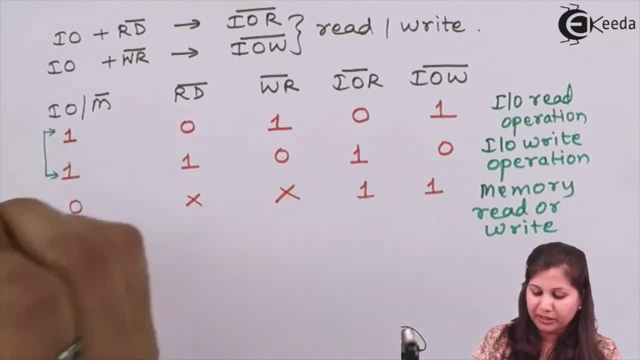 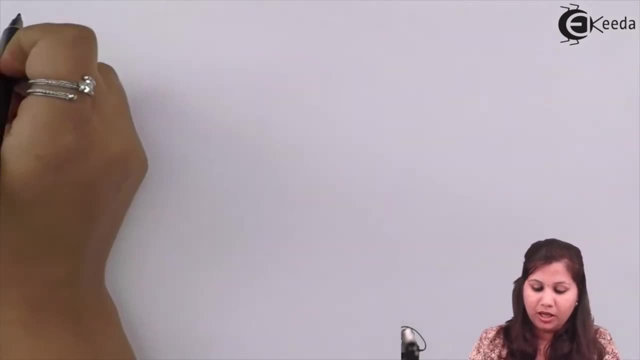 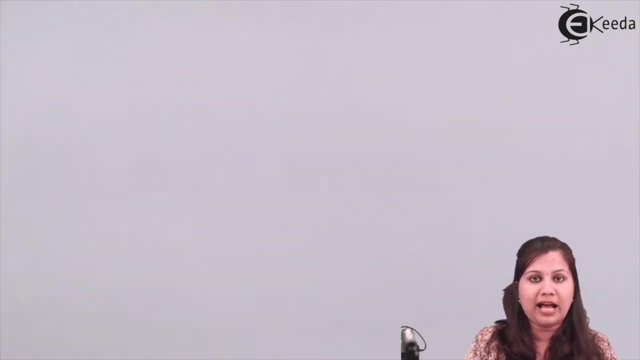 so here only these two will be the status of the control signals. Now, if we want to access the input output ports, if we want to read the data and write the data, microprocessor has to use some instructions. so for the input output devices, the two instructions. 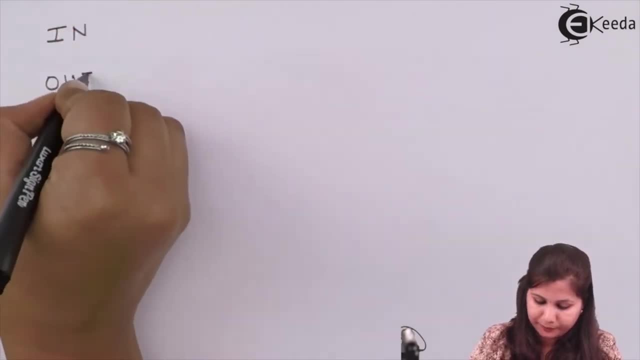 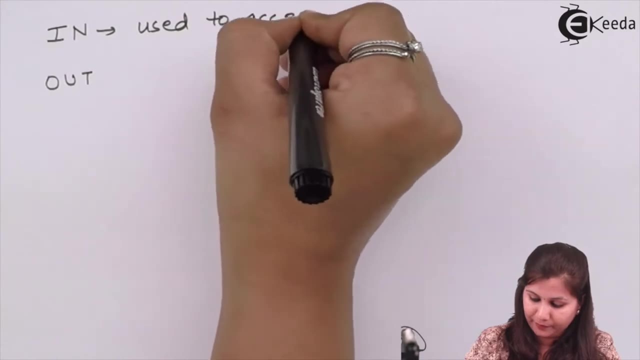 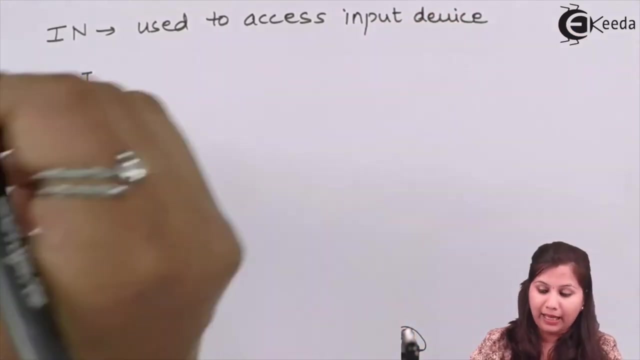 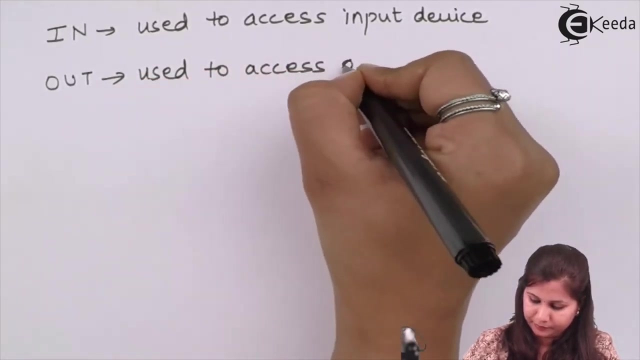 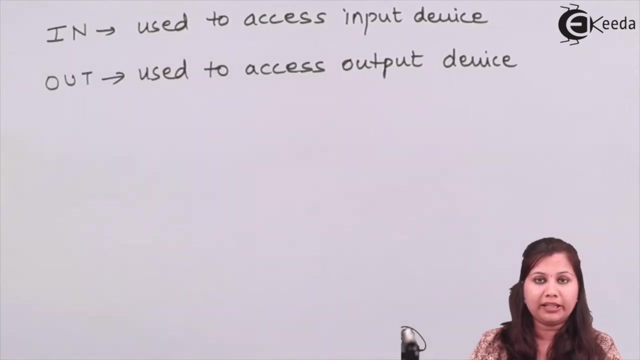 are used in and out. In is used to access the input output device, the input devices, and out is used to access the input output devices. So when in is instruction is written, whatever is the data in the accumulator, that data will be means whatever is the data at the input port, that data will be read by the microprocessor and that data 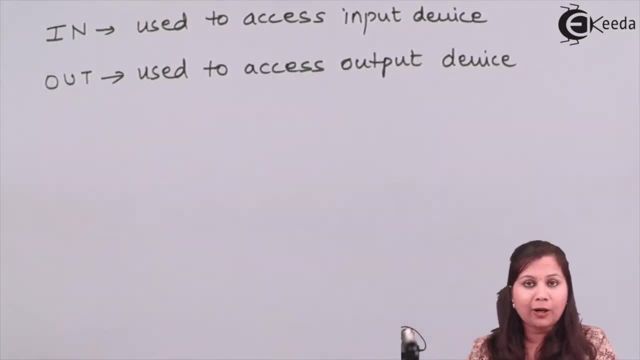 will be stored in the input port. So when in is instruction is written, whatever is the data in the data in the accumulator, When out instruction is used, whatever data is there in the accumulator, that data will be sent to the output port. okay, so out is used to access the output device. in is used. 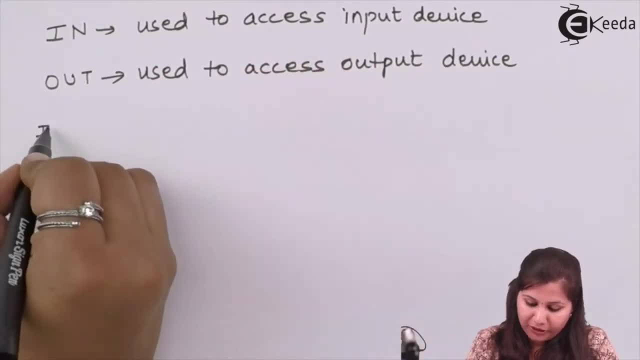 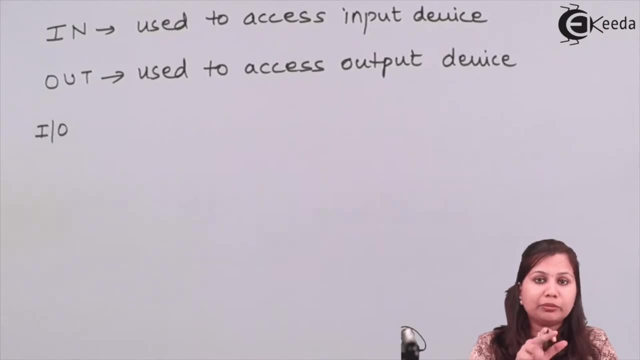 to access the input device. Now the input output devices. if we want to access them, we have to use some address so that we can locate that this input output device should be connected with the microprocessor. So for addressing the input output devices we need to connect the microprocessor with theNO in output. In is. instruction is written. 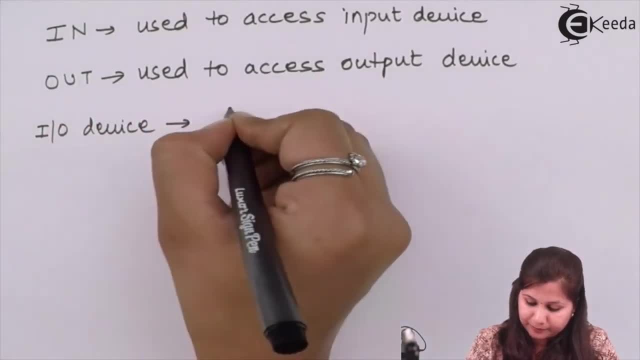 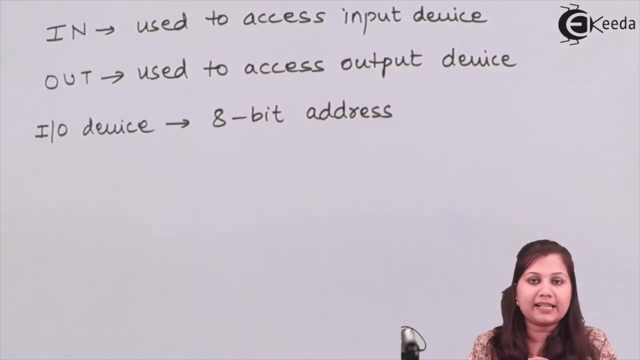 we use an 8-bit address because every input output device it is assigned a unique 8-bit address. so whenever we want to use or access that input output device we are going to provide that 8-bit address. so it is going to select that input or the output port. so an 8-bit address is there and that address. 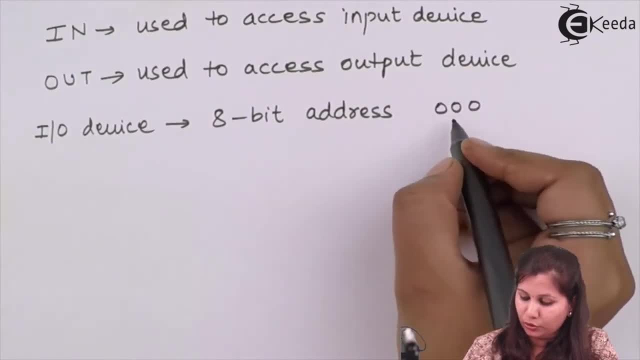 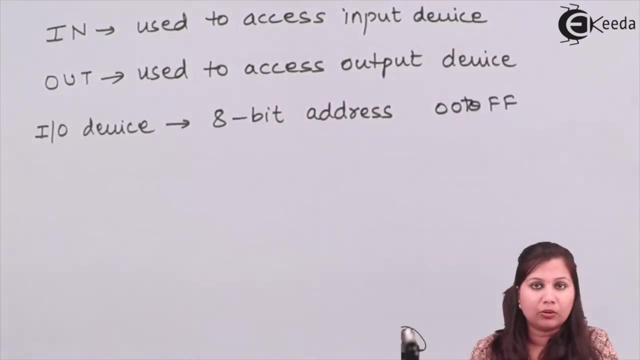 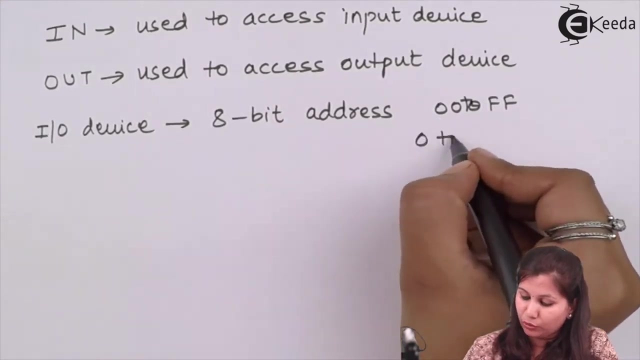 will be like: from 0: 0- 0 to, from 0: 0 to FF. okay, so here the 8-bit address range. it will be from 0 to 256, so 8-bit address can have values from 0: 0 to for. 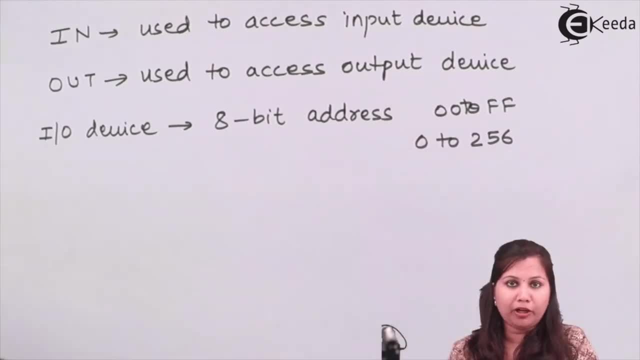 FF. so we can say that the number of input output devices that can be interfaced with an 8-bit address will be from 0 to FF. so we can say that the number of input output devices that can be interfaced with the microprocessor it can be from 0 to 256, so maximum 256 input output. 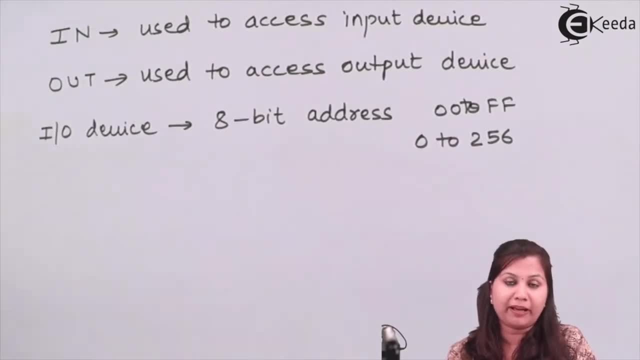 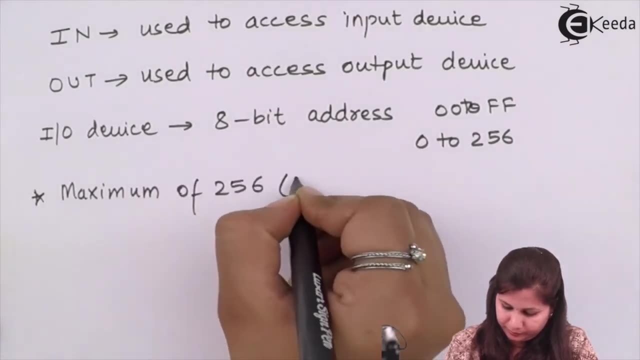 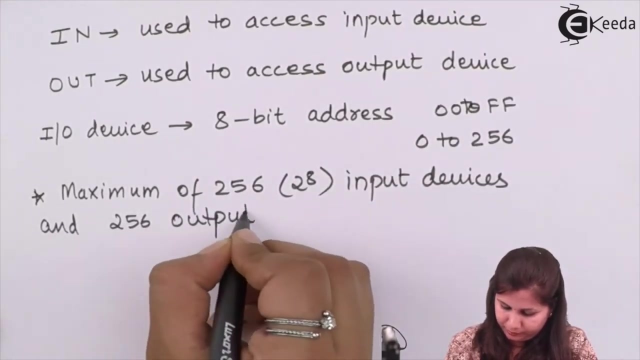 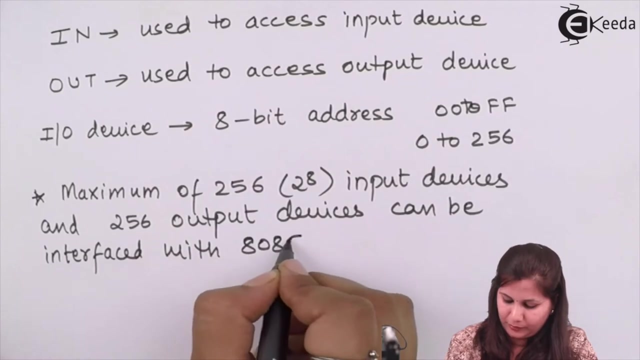 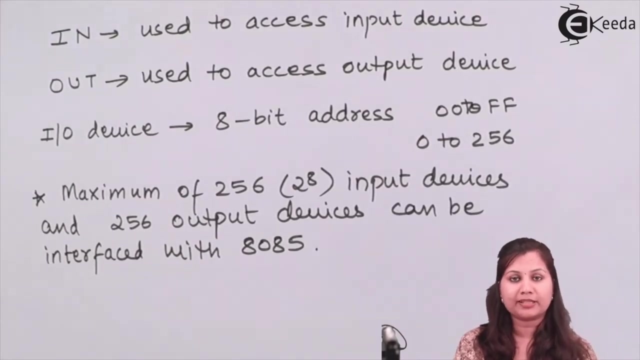 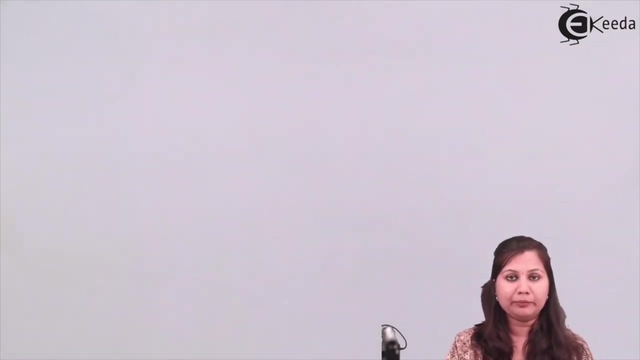 devices can be interfaced with the 8085 microprocessor at the same time. so we can say that maximum number of input output devices that can be interfaced with 8085 microprocessor is 256. okay, so in the peripheral map, input output interfacing, we are treated the input. 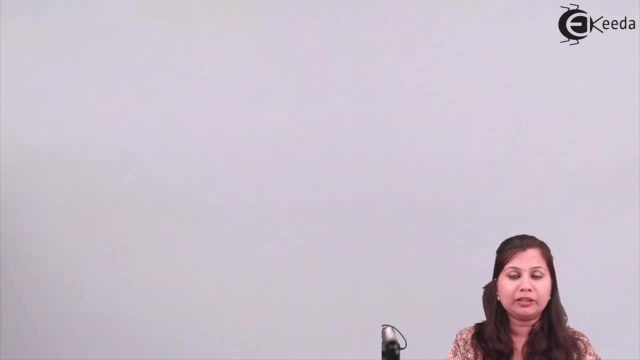 output devices different from the memory chips. they will be treated just like the ordinary input output ports. we will use the instruction in and out control. signal audio kg equal icon. I can play music by importantes outros sin vai. us facts are under control. signal standard IOR and IOW will be used to read or write the data into the input-output ports. Maximum, there will be a unique 8-bit address assigned to the input-output devices, So a maximum number of 256 input and output devices. they can be interfaced with the microprocessor. Now let's come to the second type of input-output interfacing, which is the memory-mapped input-output interfacing. 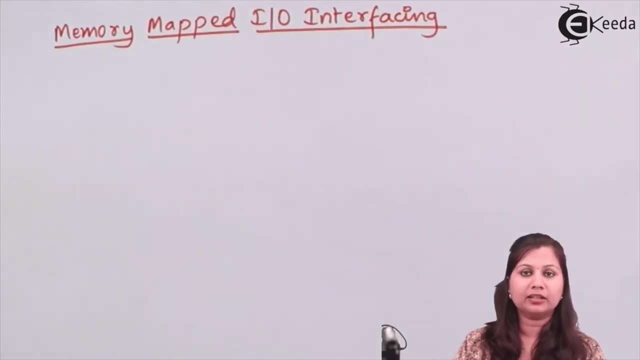 So in the memory-mapped input-output interfacing- the input-output devices- they are treated just like the memory chips. So whatever interfacing technique is used to interface the memory chips with 8085, same technique will be used for interfacing the input-output devices. 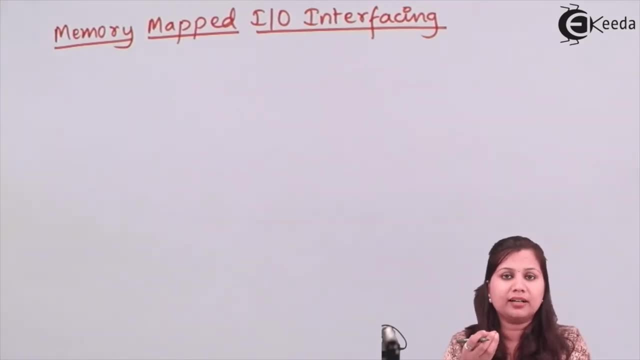 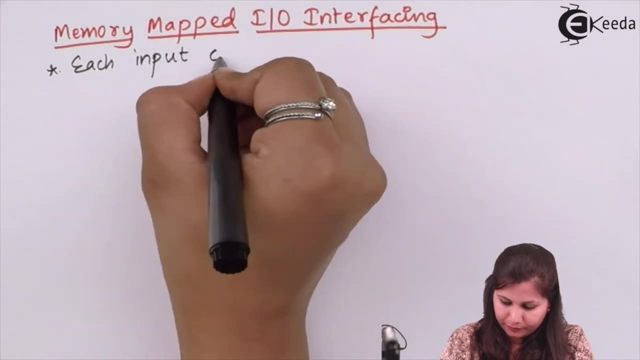 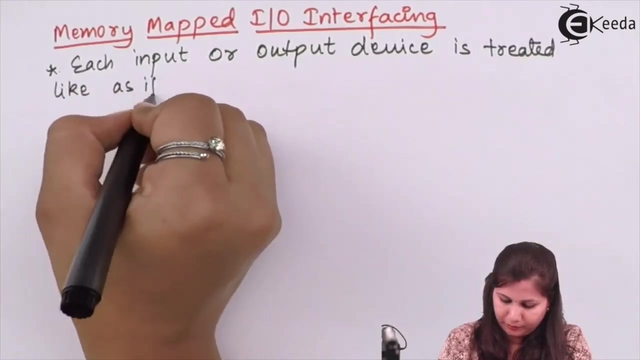 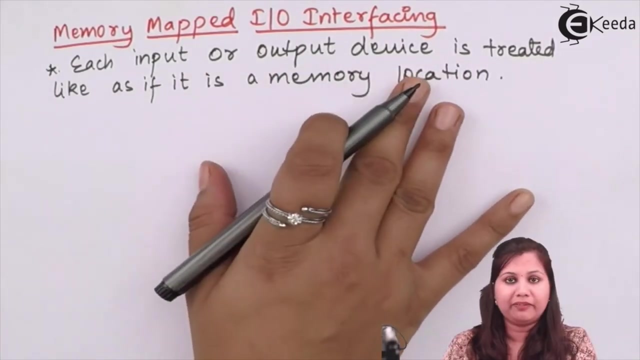 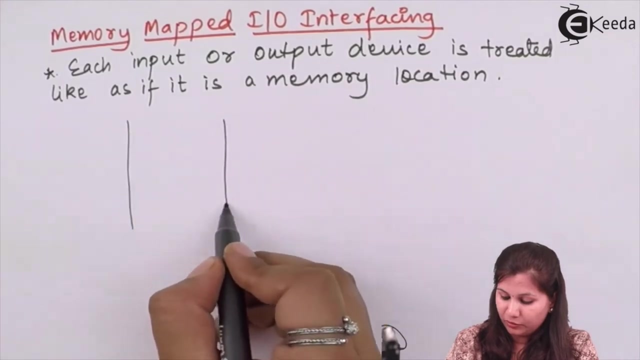 So they will be just like the memory locations in the memory of the microprocessor, So each input or the output device it is treated like as if it is the memory location. So suppose this is the memory of the 8085 microprocessor. 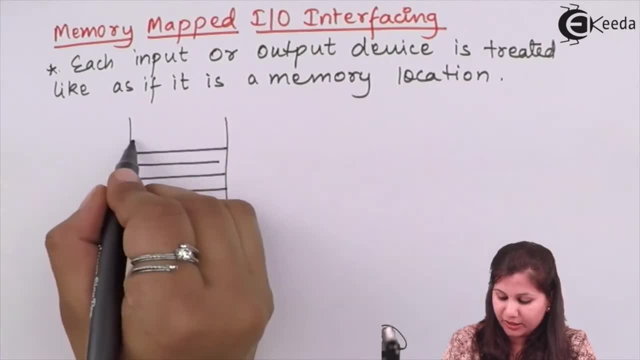 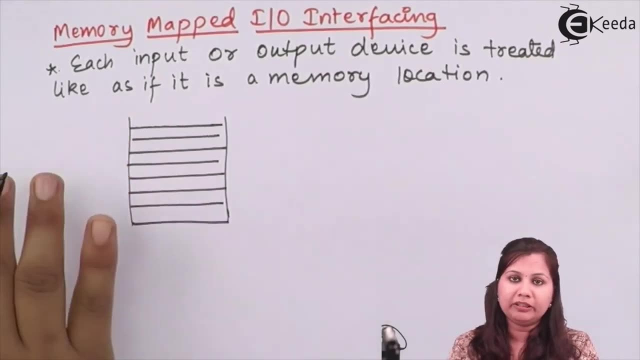 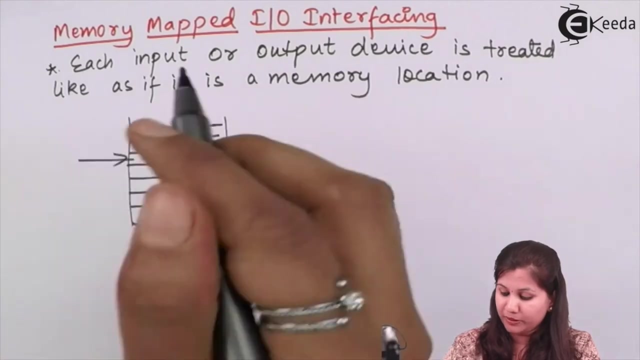 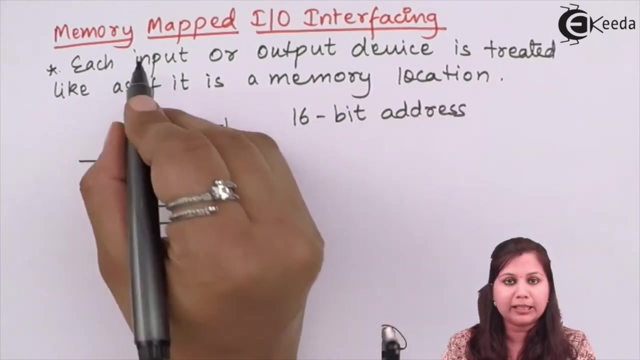 In that memory we are having the different registers and or we can say, memory locations are there. So input-output devices, they will be treated also like a memory location. So for addressing a memory location in 8085 microprocessor we use a 16 bit address. so same 16 bit address will be used for addressing the input output. 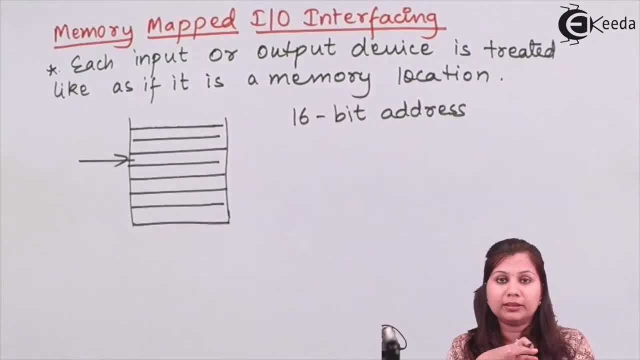 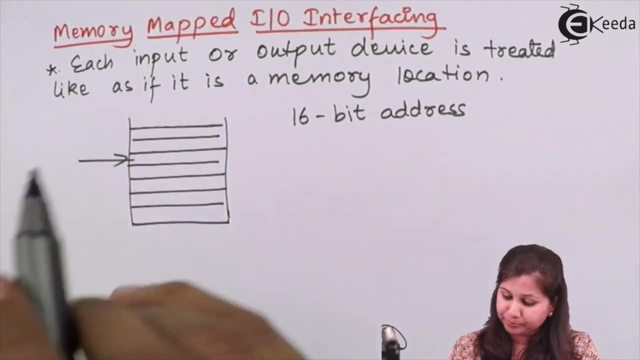 devices also. so in the case of in the peripheral mapped input output interfacing, we studied that 8 bit unique address is assigned to the input or the output devices, but here the address is a 16 bit address. okay, now there. we studied that the control signals are the input, output read and. 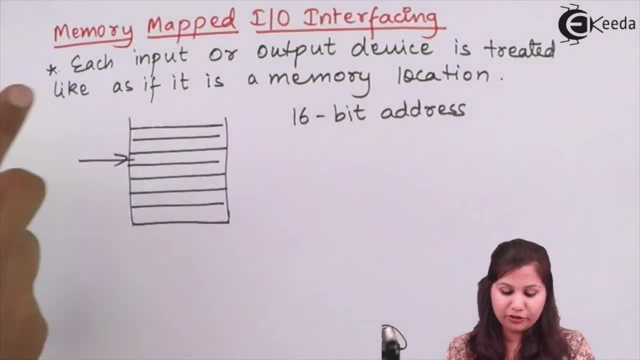 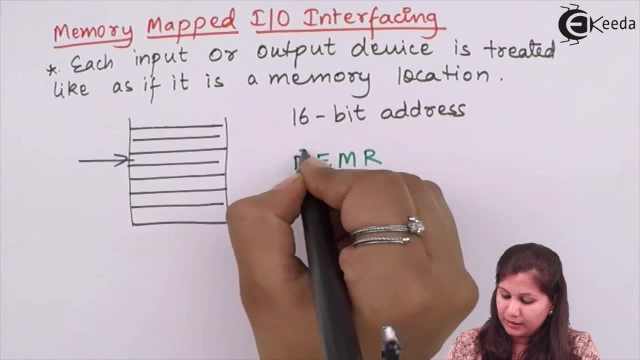 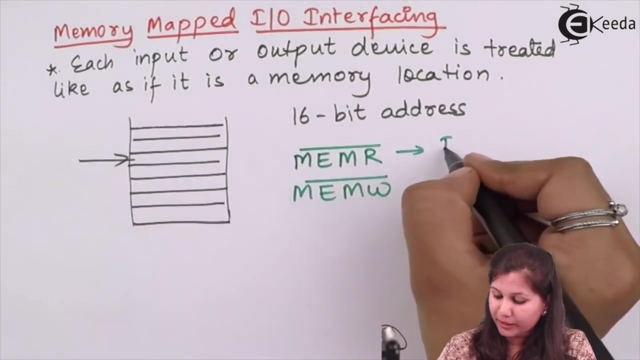 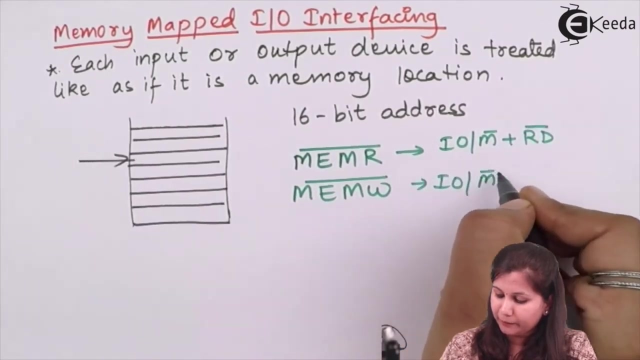 input output right now here because it is a memory location. so control signals will be changed. it will be M E M R and M E M W. and how these signals are formed by the combination of input output memory plus the read and input output memory plus run. so when this input output memory 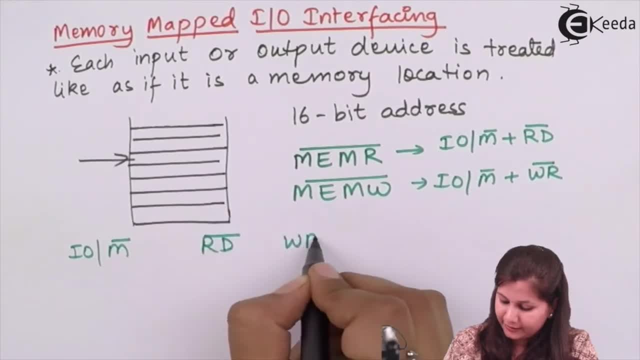 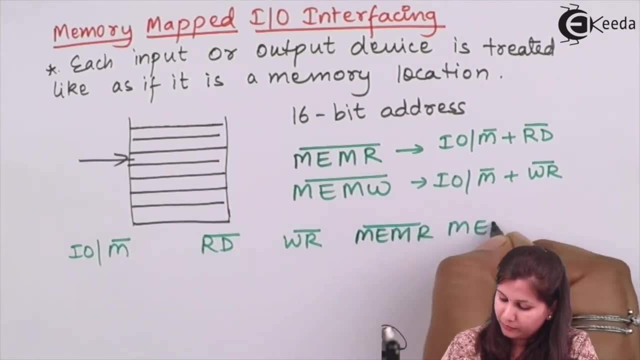 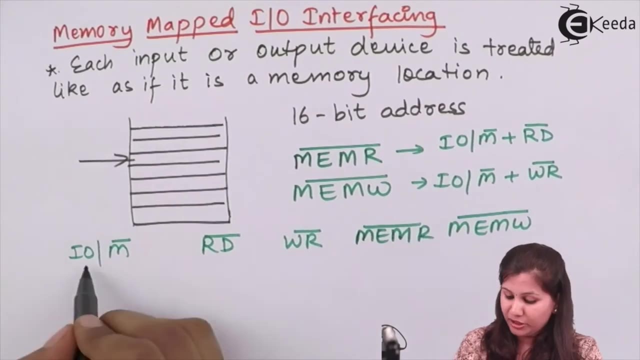 is set to the input output memory, then the input output memory is set to the input output memory. signal: read signal, write signal. and we are having M E M W R and M E M W. what will be their status? what type of operation will be performed for a memory operation? this signal has to be 0, then only the 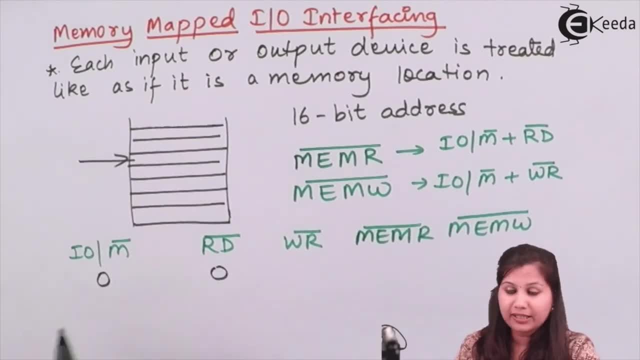 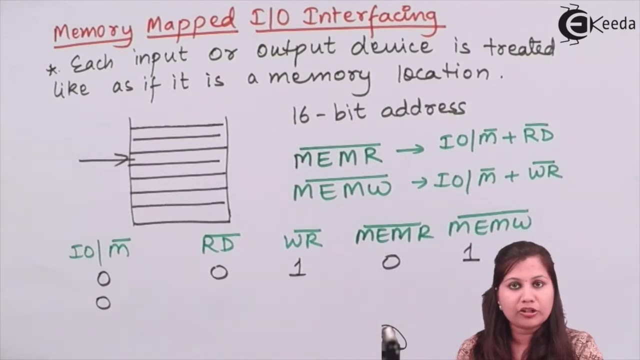 memory operation will be activated. now when read is 0 means it is activated. then M E M R is activated. the operation performance will be 0 and the memory operation will be activated. then the memory operation performed will be a memory read operation. others will be are at logic 1 when, again, this is at logic. 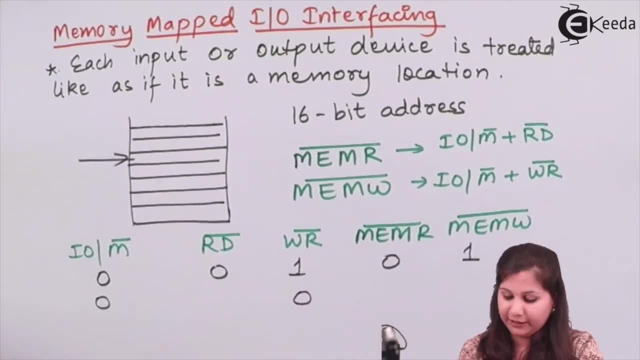 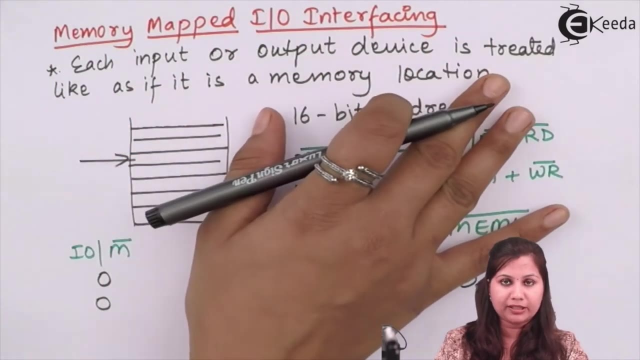 0 and write is at logic 0 means it is activated. then M E M W will be activated and the operation will be a memory write operation. so this will be the status of the control signals in the memory map input output interfacing. so for M E M R is used to read the data from the input output memory. 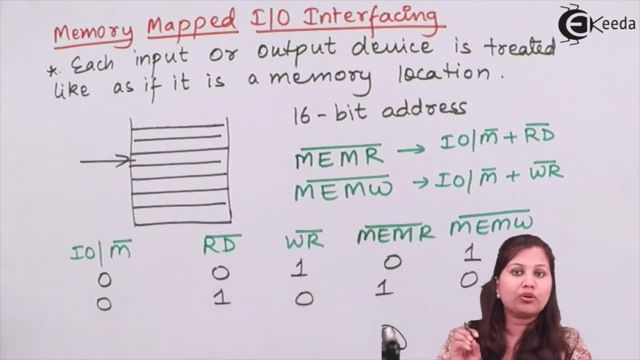 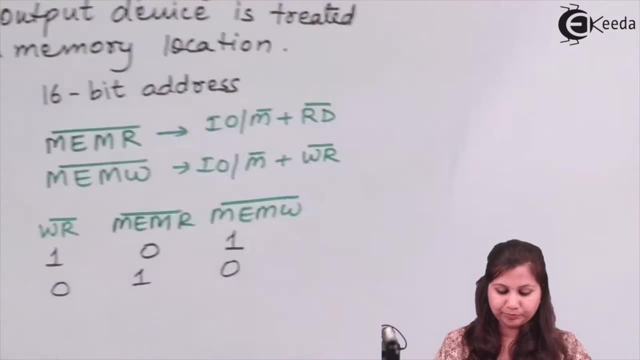 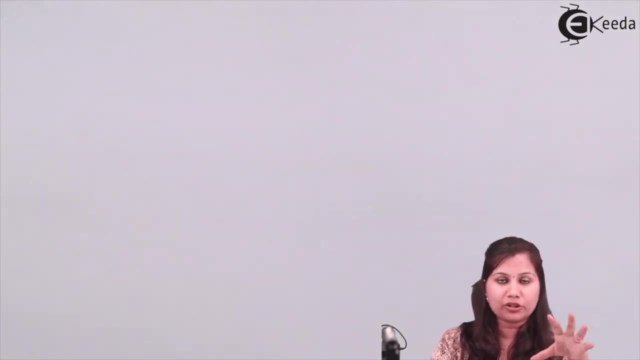 from the memory location and M E M W is used to write the data into the memory location, or we can say the input output devices. now in the peripheral map, input output interfacing, we were using the in and out instructions to read and write the data. here also microprocessor will use. 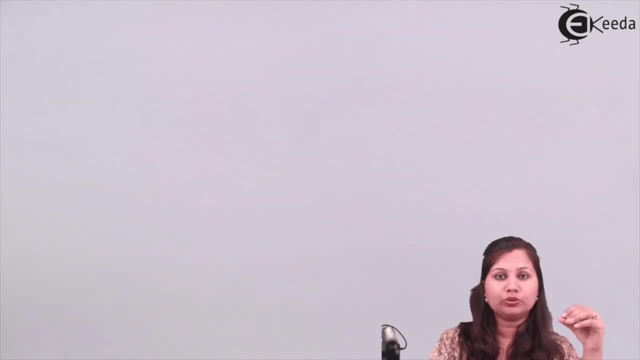 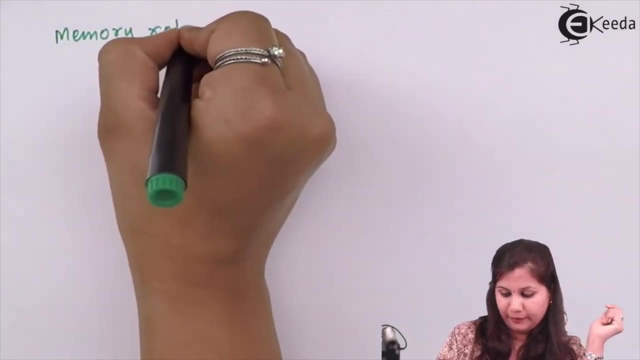 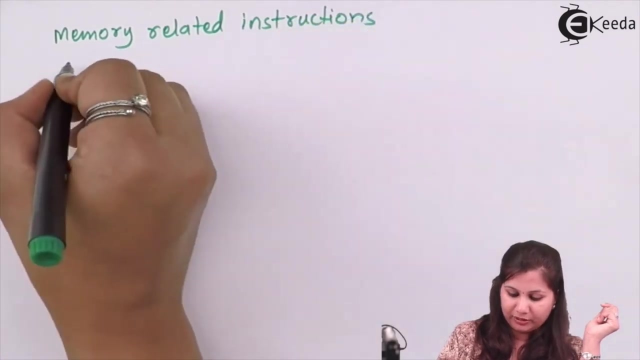 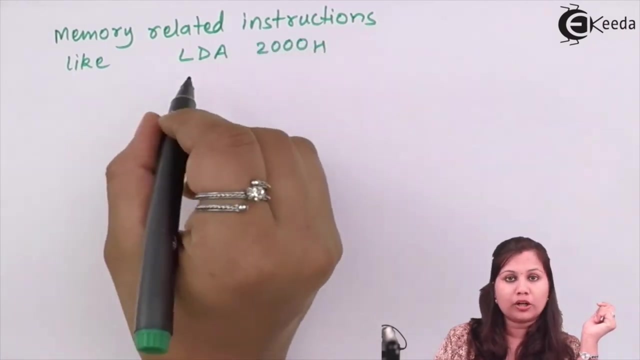 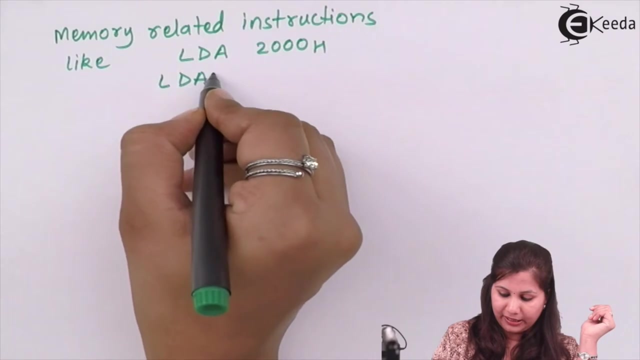 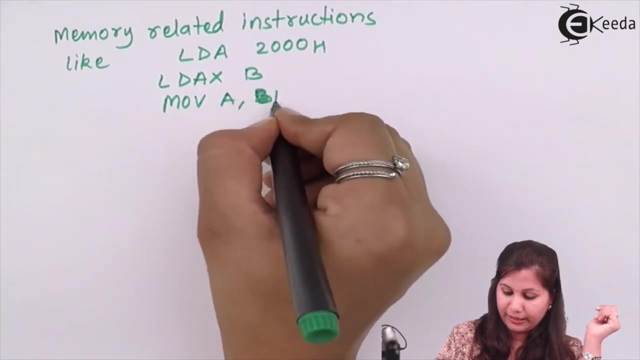 the instructions, But those instructions are related to the memory, so memory related instructions are used like we are having the LDA 2000 edge, so accumulator is loaded with the data at the memory location 2000. again we are having LDA X B. we are having move a comma B, sorry, a comma M. 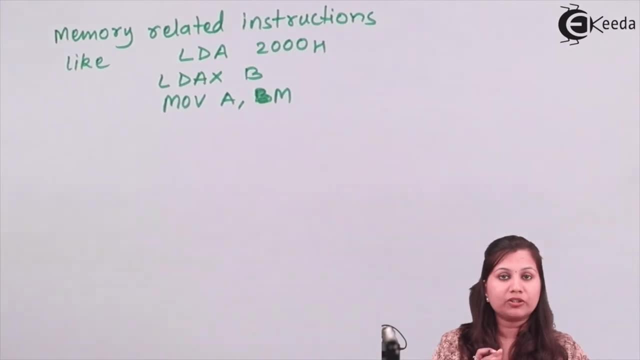 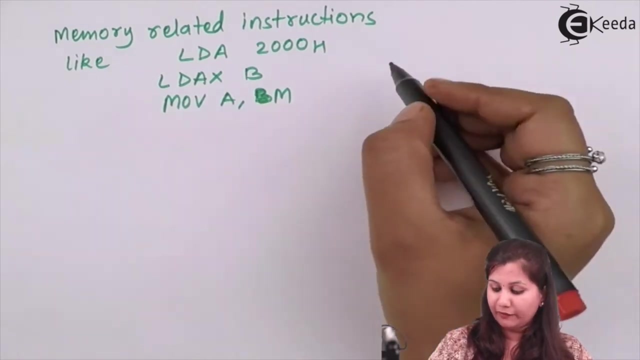 okay, so all the instructions which are related with the memory location. those instructions can be used for reading and writing the data, and here the address is the 16-bit address. now, because the the input output devices, they are treated just like a memory location. so in microprocessor 8085. 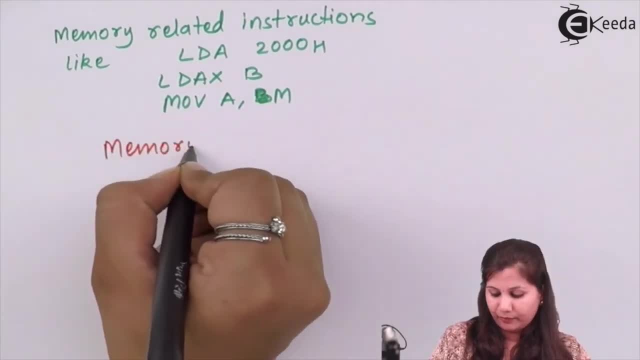 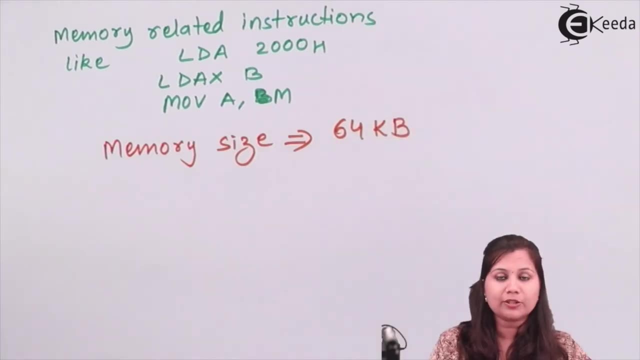 the total memory size is 64 kilobytes. the memory size of the 8085 microprocessor is 64 kilobyte. so this memory size, the 64 kilobyte, it is shared with the memory of the microprocessor also and by the input output devices also in the memory map interfacing because they are also like memory. 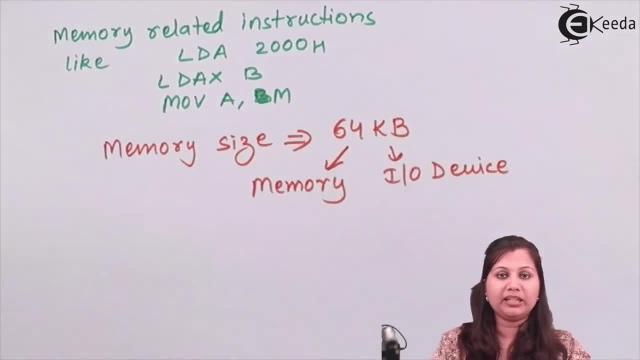 location. so all the 64 kilobyte of memory. it is divided between the memory and the input output devices. but this is not the case in K, in the peripheral map input output interfacing. they are the 64 kilobytes of memory. it is completely shared by the memory of the microprocessor. 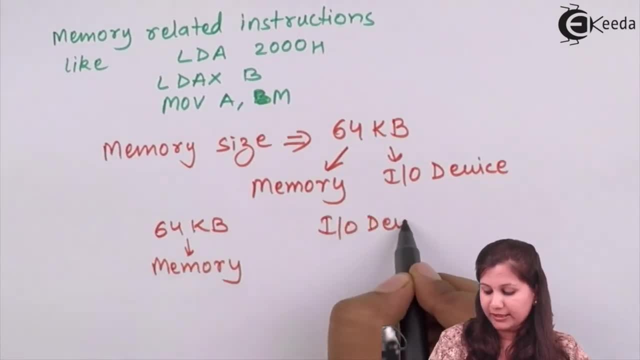 the input output devices. they will have the separate. they are treated as the input output devices only, so they are not going to share this 64 kilobytes of memory. so we can say that in the memory mapped input output interfacing the memory size used by the microprocessor, it is reduced okay. 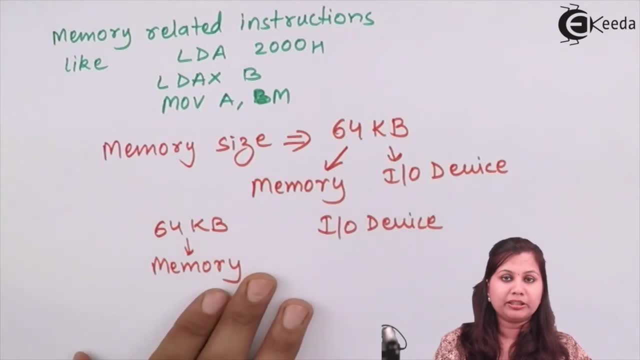 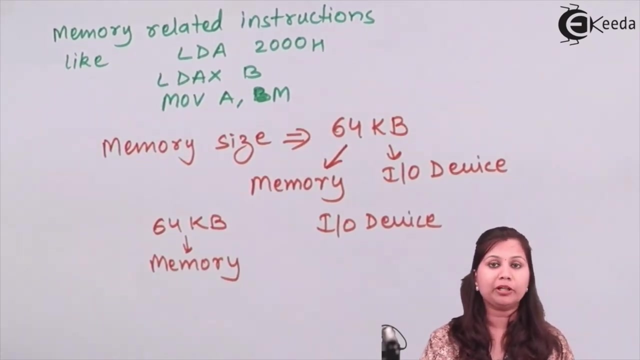 whereas in the peripheral map input output interfacing complete 64 kilobyte of memories. so this is the. these are the two types of input output interfacing. well, that means in these two ways, the input output devices, they can interface or they can communicate with the 8085 microprocessor. 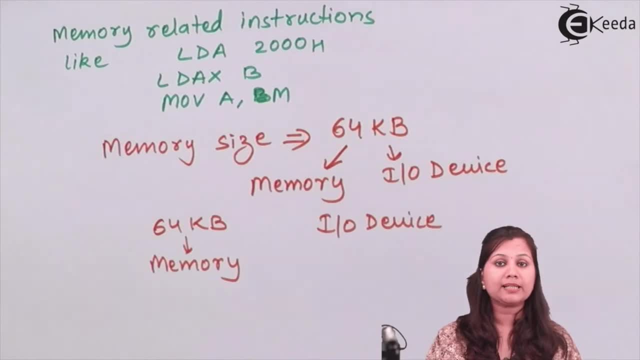 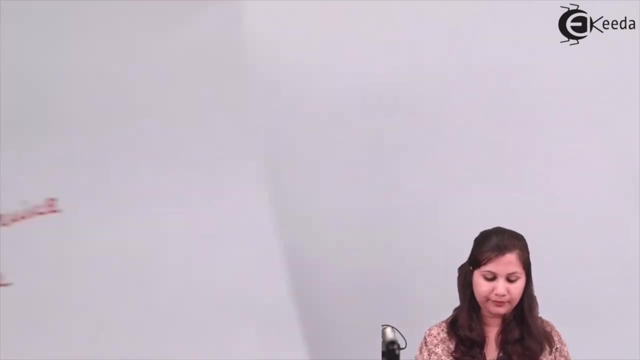 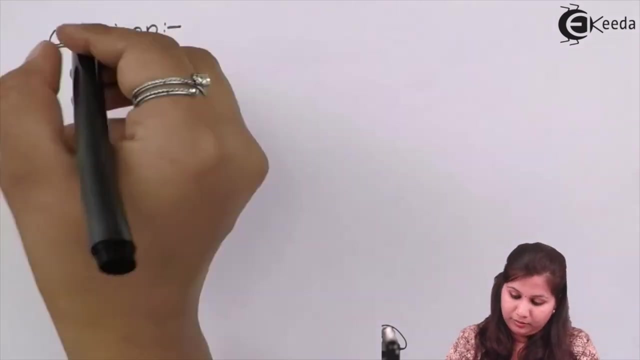 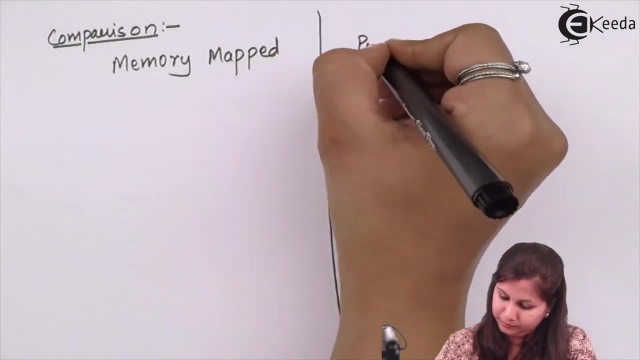 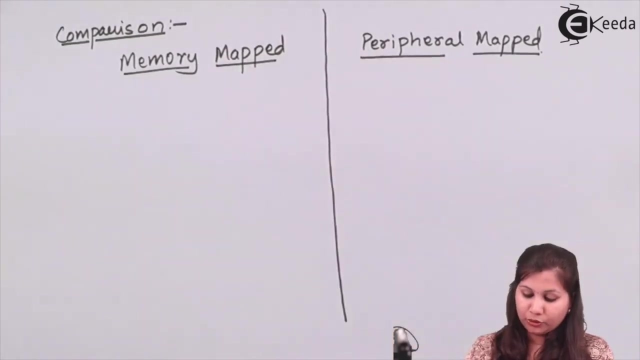 now, after studying these two types, let us compare the two types of interfacing. so let's study the differences between them. so the first difference between the two types of interfacing is that in memory map we are having the addresses for the input output devices as 16-bit addresses. 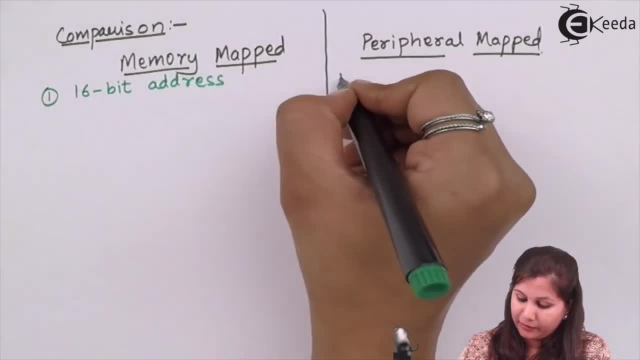 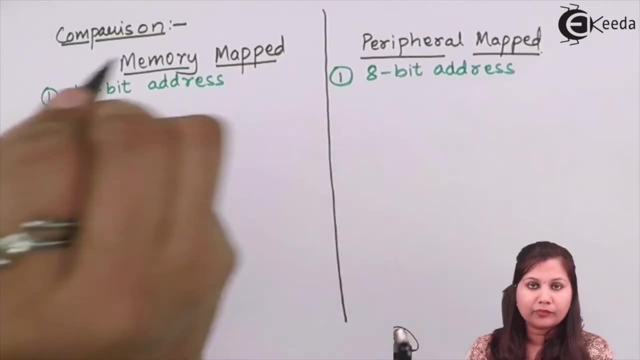 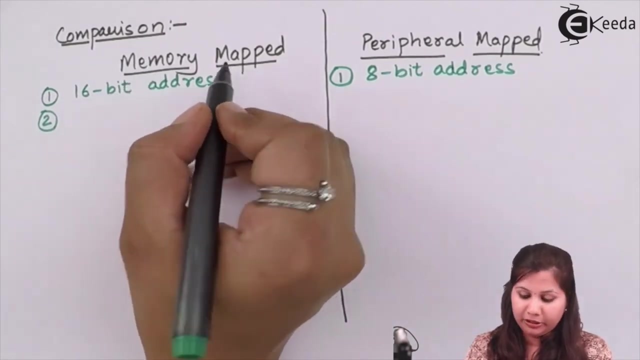 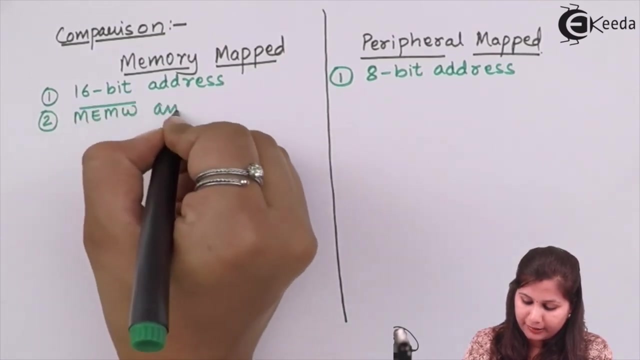 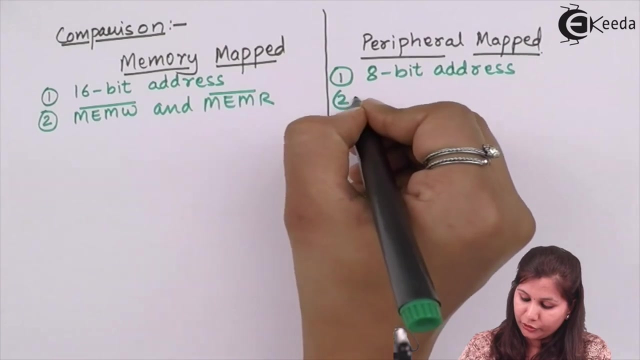 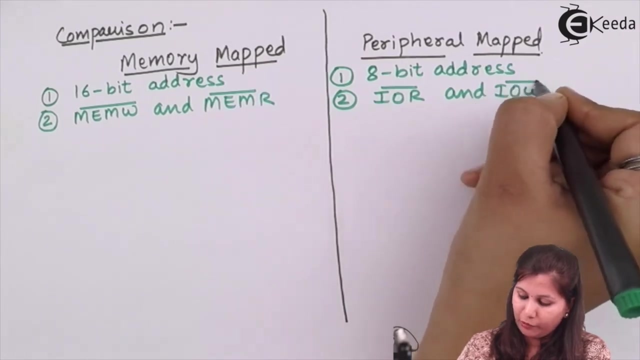 and in peripheral map we are having the addresses for the input output devices as 8-bit address, so addressing is changed. second difference is in the memory mapped interfacing we are using the memory control signals, that is, mem w and mem out, whereas in peripheral map we are using the input output read and IOW input output write. 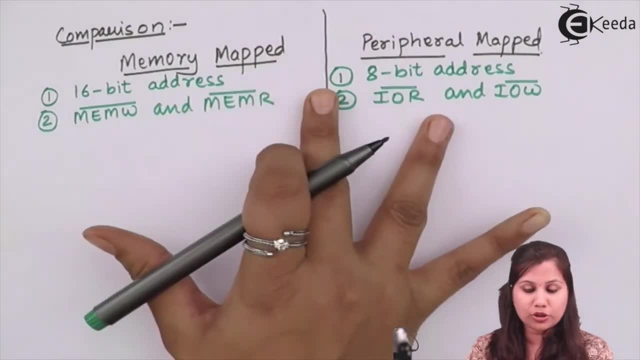 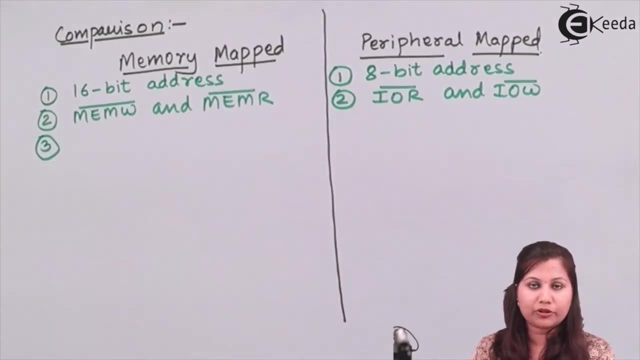 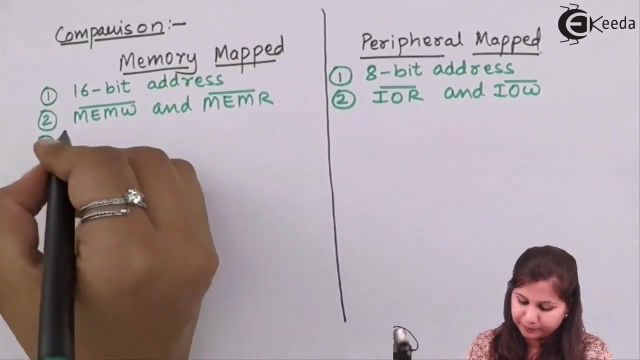 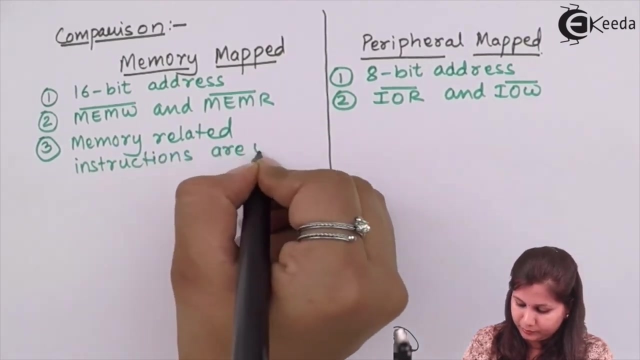 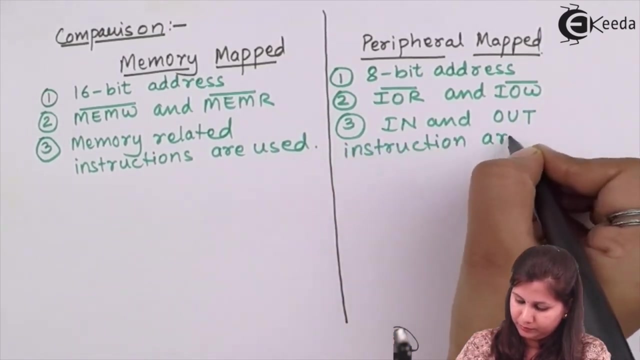 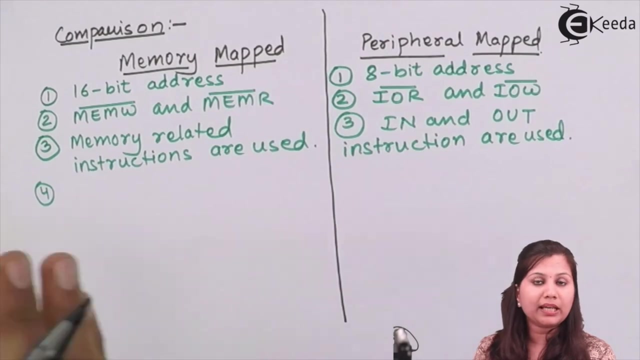 control signals. so control signals are also changed. third, in memory map we are using all the memory related instructions for reading and writing the data. in peripheral map we are using the in and out instructions. you in memory map interfacing. the data transfer is taking place between any 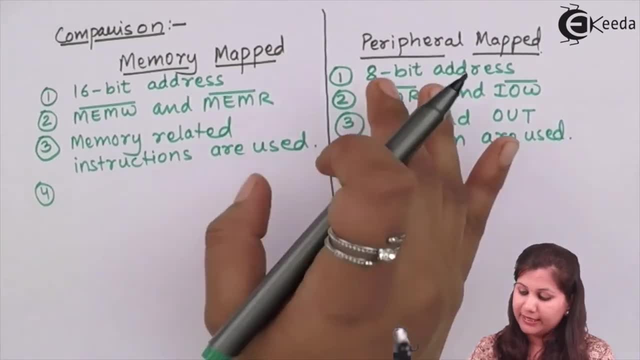 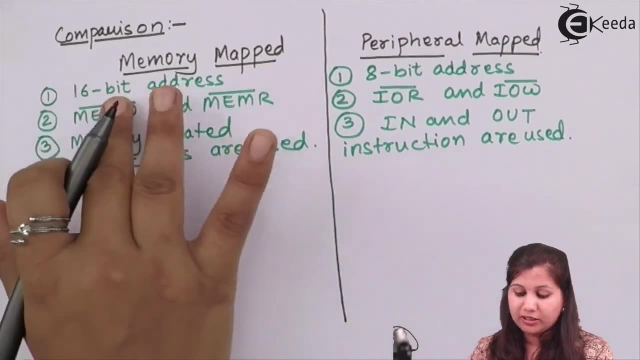 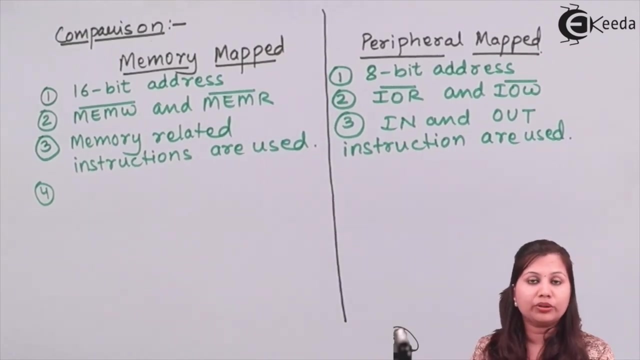 register and the input output, whereas in the peripheral map the data transfer is taking place between the accumulator and the input output device, because here we are having the, we are using the input output device, treating them like as a memory location. so data transfer will be between the memory register and the input output. 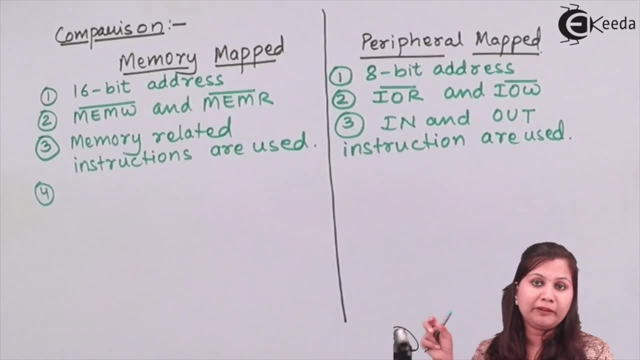 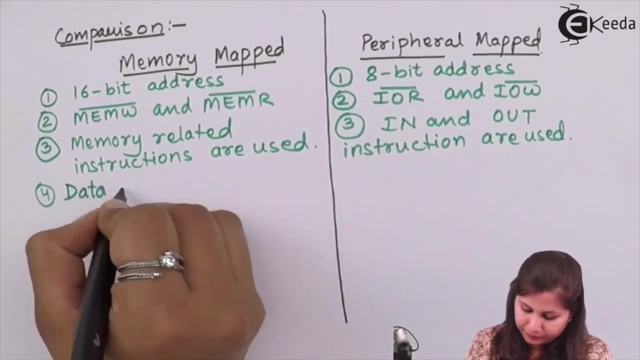 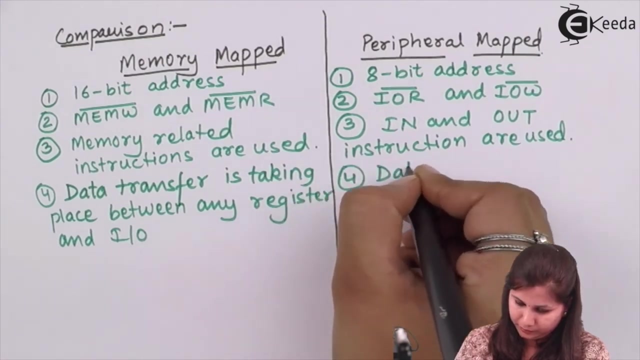 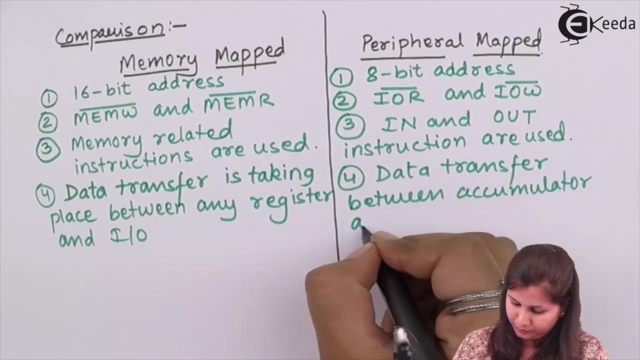 devices, whereas in peripheral map all the data will be first stored in the accumulator, then only it will be transferred to the input output device. so reason for setting: the data transfer is being managed by memory map interfaces based on the directions and hence obligations of both edition books. 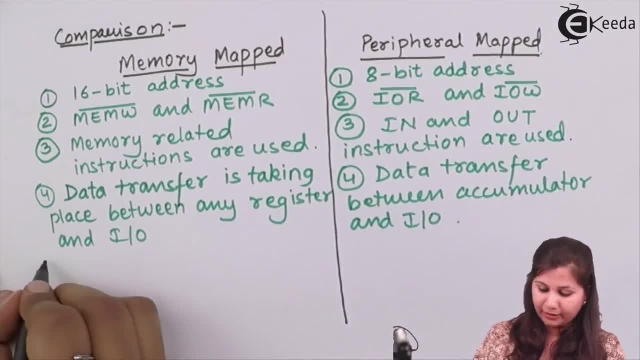 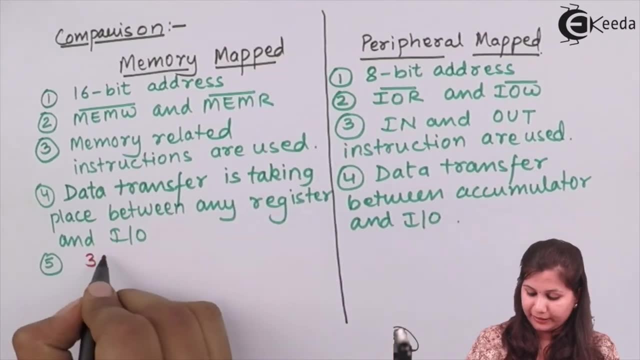 and keep it simple. now in memory map interfacing, as we are using the memory related instructions. so all the memory-related instructions. they are three byte instructions, so they are going to use more memory in the current e-book, but just for now this is enough for that functions. order is available as per internet we are using in this instance. so are we gonna add some other objects here? day? 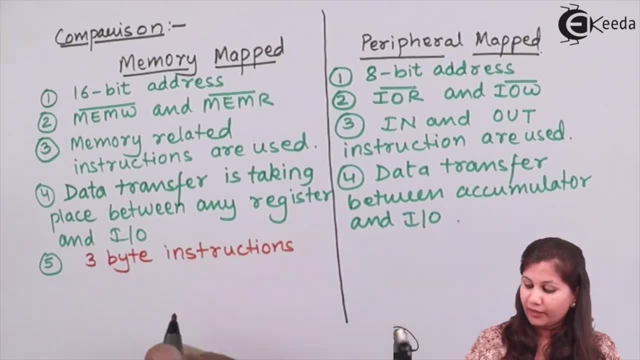 in the microprocessor for their storage, whereas in and out instruction they are the two byte instructions only. so two byte instructions they will use less space as compared to three byte. so memory map instructions, memory related instructions, they are going to use more space, whereas peripheral map the 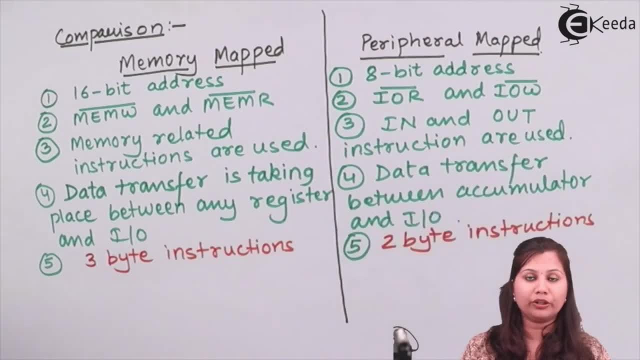 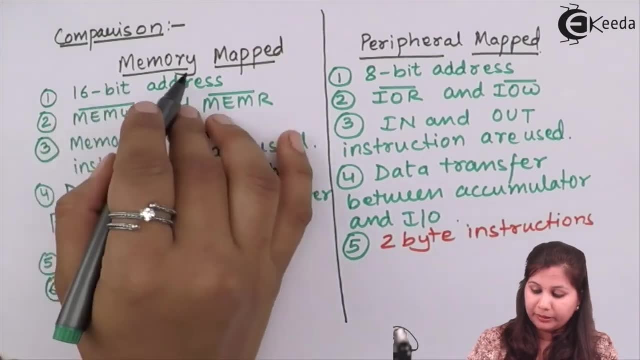 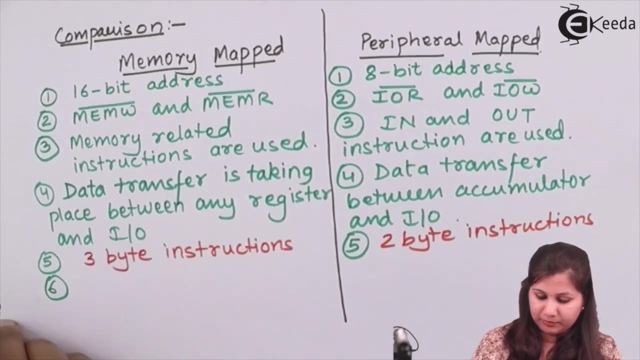 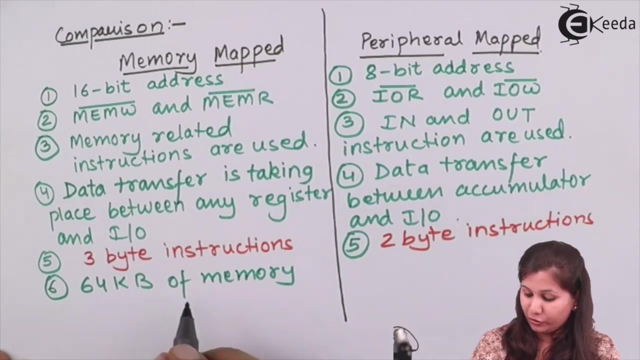 instructions, the in and out instructions. they are going to use less space now in memory map because we are having 16-bit addresses are there. so the complete the number of input output devices it can use complete 64 kilobyte of memory because we can say that the 64 kilobyte of memory is shared between input output. 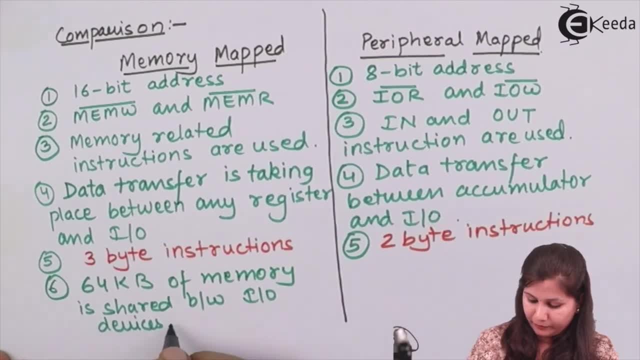 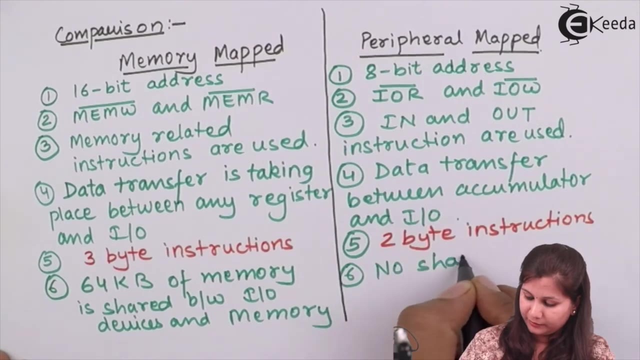 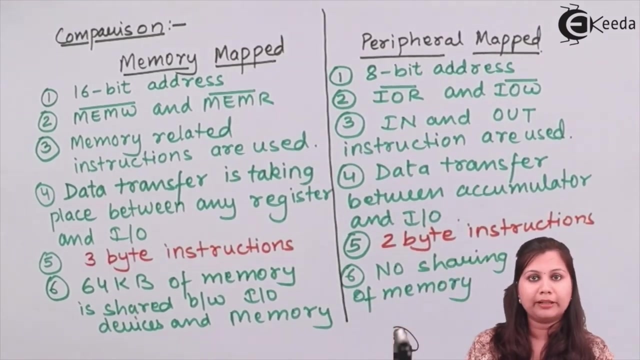 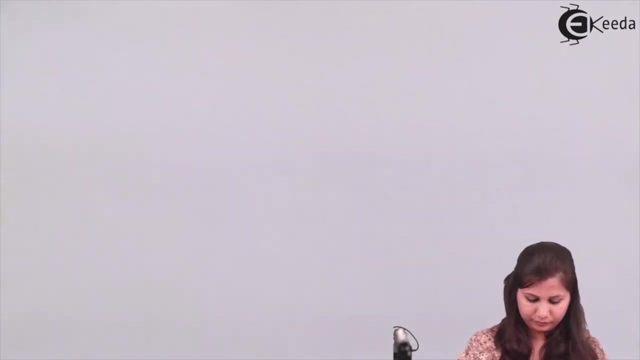 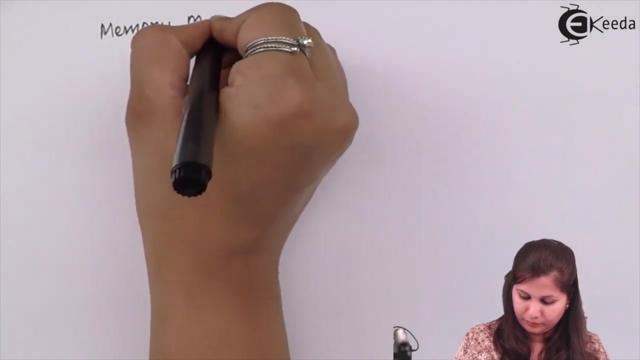 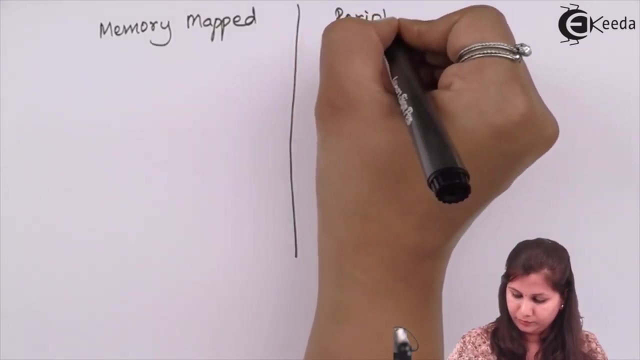 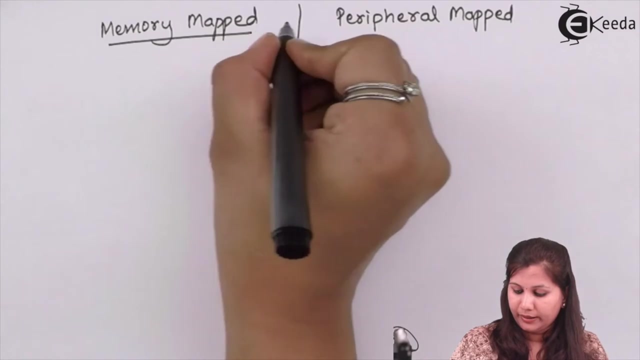 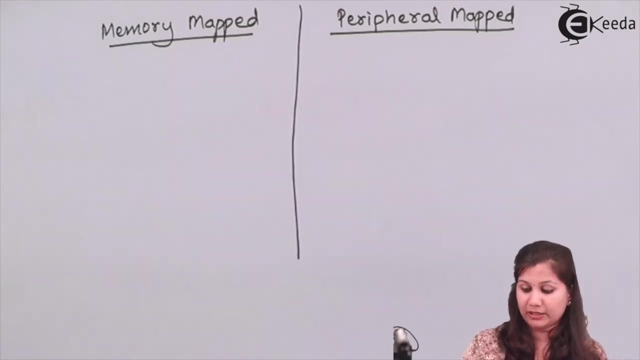 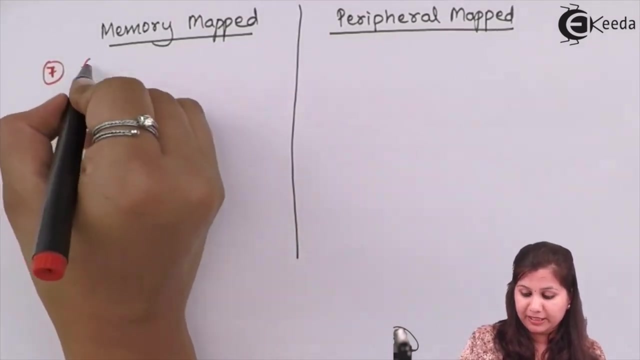 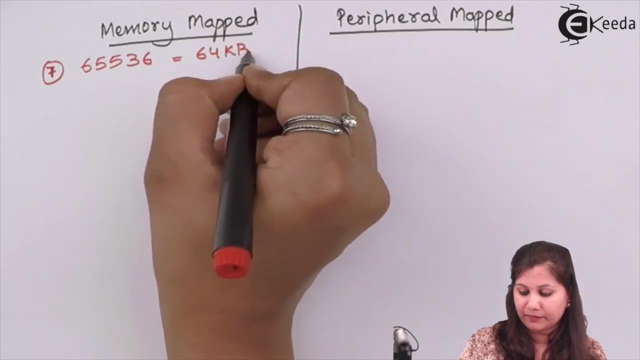 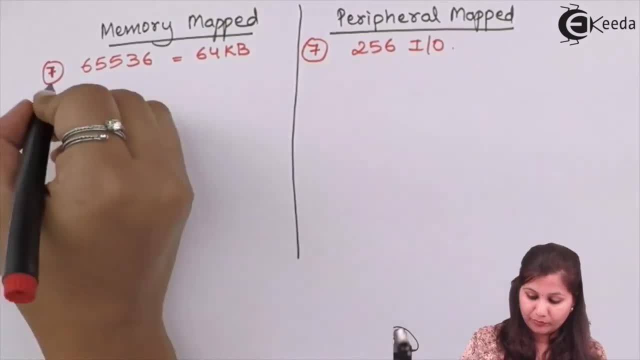 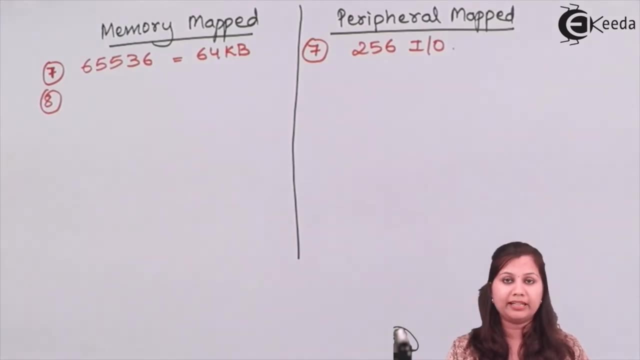 it is equal to 64 kilobytes, whereas in peripheral map interfacing the maximum number of input input interfaces is 256 456. because the memory map too, input output interfacing- it is using memory related instructionWe're using memory related instructions- техyak Ho Christmas 3, closer instruction, so more hardware is require for decoding those instructions, whereas in peripheral map, because we are having only 2 byte instructions, We're using memory related instructionμεhr局 identifier. we cannot decode that as Hyacinth. so now I am going to show it the How to use YCM & Gaiaalsver and support your current Mixi. 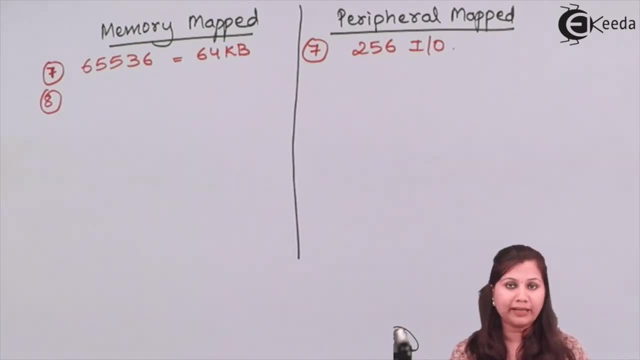 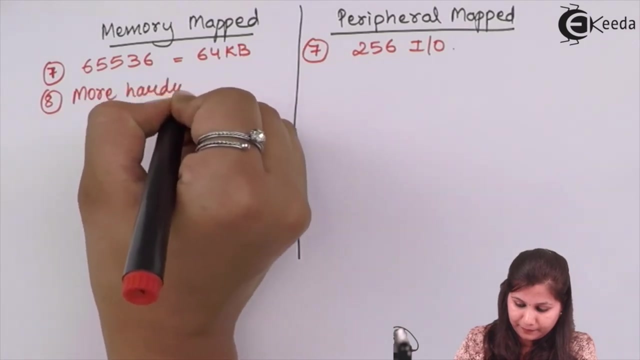 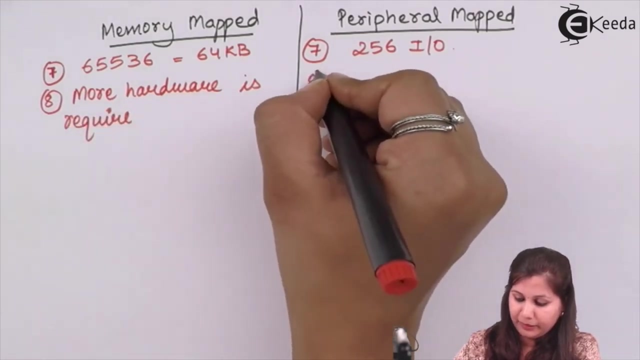 whereas in peripheral map, because we are having only two byte instructions there will require that two byte instructions. they will require less as space and also less circuitry will be. less as space and also less circuitry will be. so here we can say that more hardware is required and in peripheral map less. 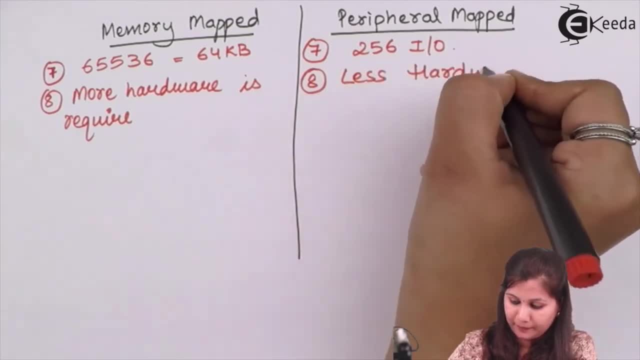 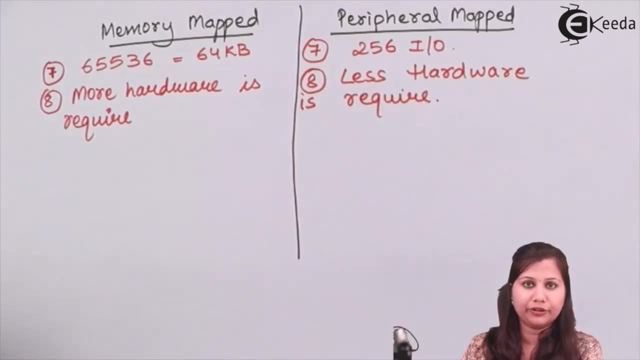 hardware is required or we can say that the complexity of the circuit is reduced because your memory map the circuit will be more complex as compared to the peripheral map interfacing. now in memory mapped all the arithmetic and logical operations. they are directly performed on the input output data, whereas in 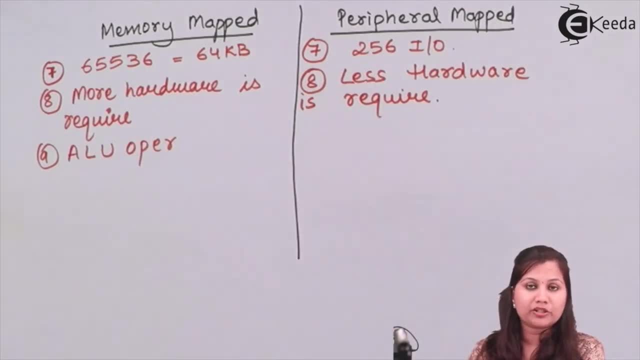 peripheral map with the all the arithmetic and logical operations. they are performed indirectly on the data, because first the data has to be stored in the accumulator and then the data will be performed or the operation will be performed with the accumulator. okay, suppose we want to add two numbers. one number is there with the microprocessor and 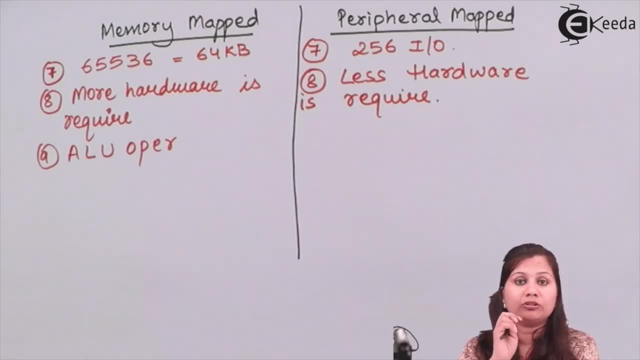 one number is stored in the input output devices. now that number has to come into the accumulator and then the addition of the two numbers will be performed, whereas in memory map the number is stored in the memory locations only. so we need only to add the two memory locations, then we. 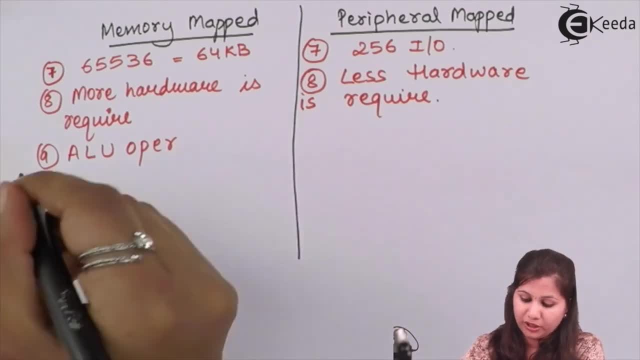 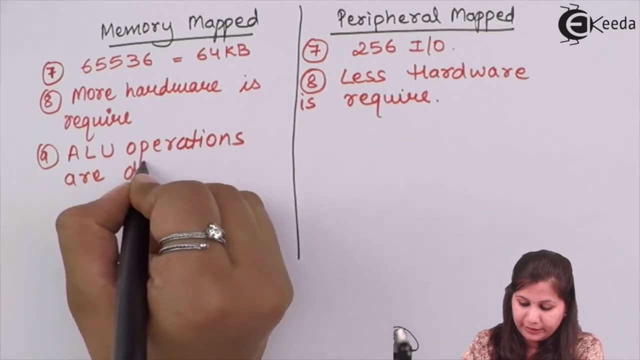 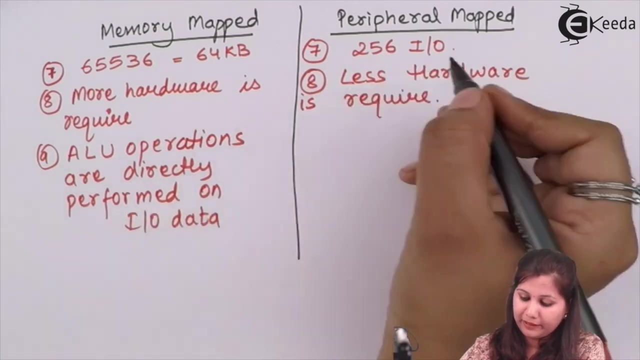 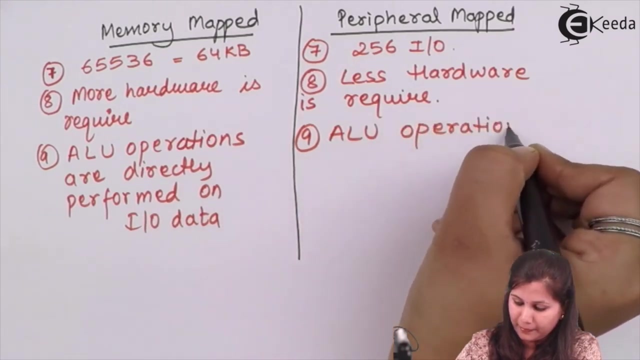 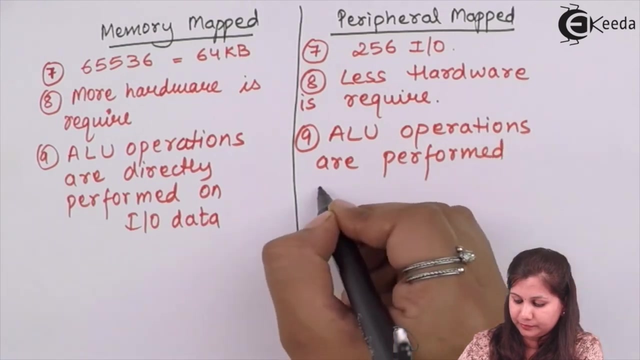 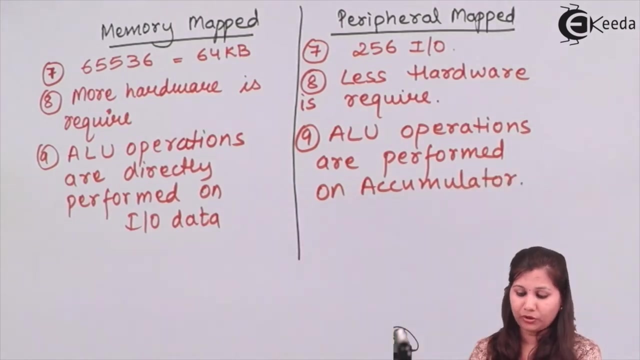 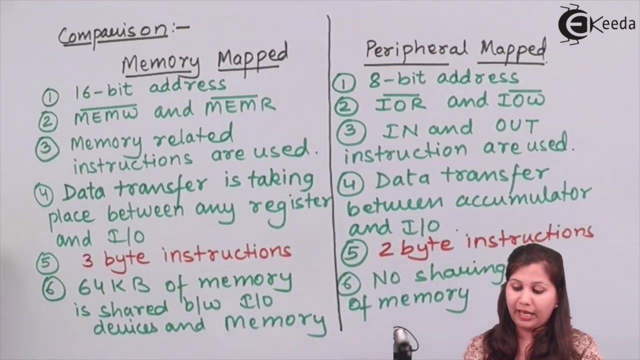 can perform the addition operation. so your ALU operations are directly performed on the data, whereas in peripheral map, the ALU operations are are performed on accumulator. okay, so these are the differences between the memory map and the peripheral map. input output interfacing- we have seen that in 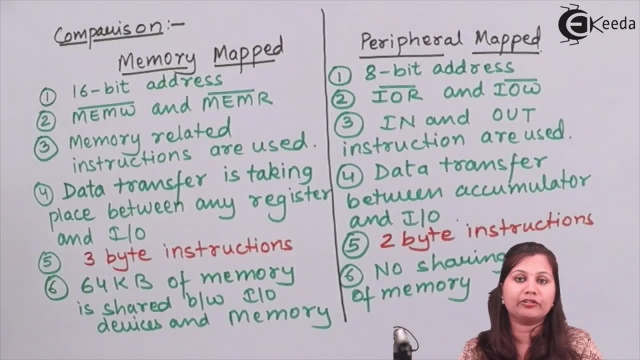 memory map interfacing the input output devices, they are treated just like a memory location, whereas in peripheral map input output interfacing the input output devices, they are treated like the ordinary input output ports and the instructions and operations related to the input output they will be performed. 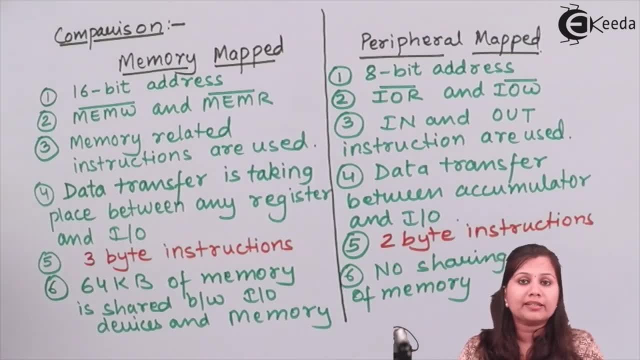 in this type of interfacing. so here in this video we studied the interfacing of input output devices with the 8085 microprocessor. we studied the two types of input output interfacing, and in the last video we studied the two types of input output interfacing. and in the last